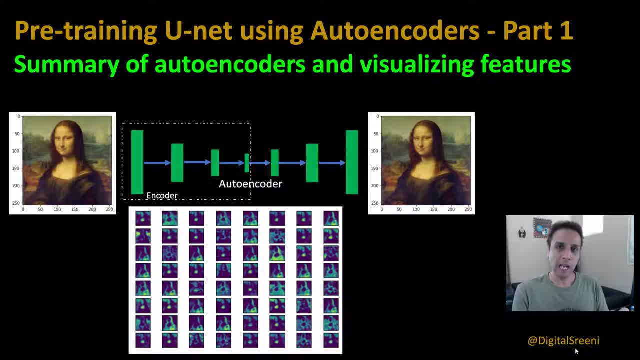 weights, meaning they probably already know how to detect certain edges, or you know rounded features and so on, and then you go from there. So what I'm proposing here is very similar to that, except instead of using pre-trained weights from ImageNet and VGG or something I'm talking about using your. 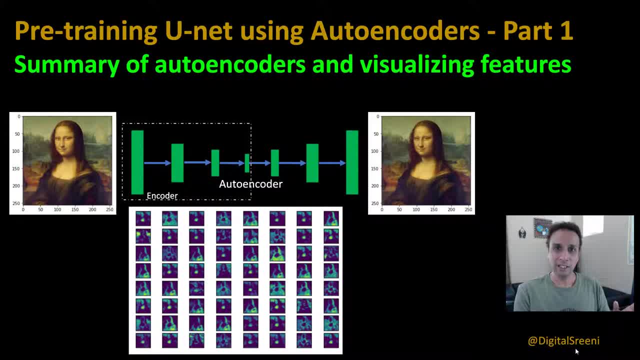 own auto-encoder on your own data and then generating weights. Okay, so what do I mean by that? Now you have a, let's say, hundreds of electron microscopy images, or some images, right, And you know that in future you'll be keep working on these, and then you're trying to train a model. It makes sense for you. 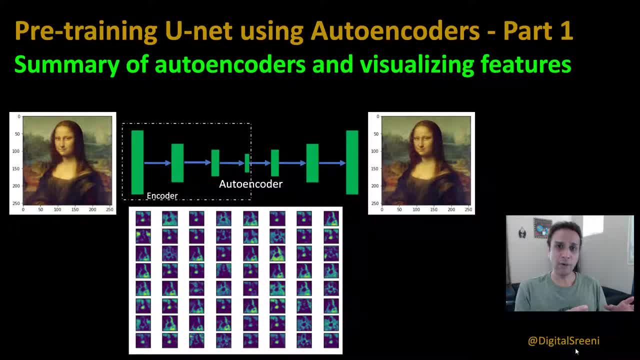 to put some time ahead of time in generating the initial weights. Instead of starting with random weights, start with weights where it has been trained on your own data. This is exactly what we are talking about Now. how do you generate these weights if you don't have the 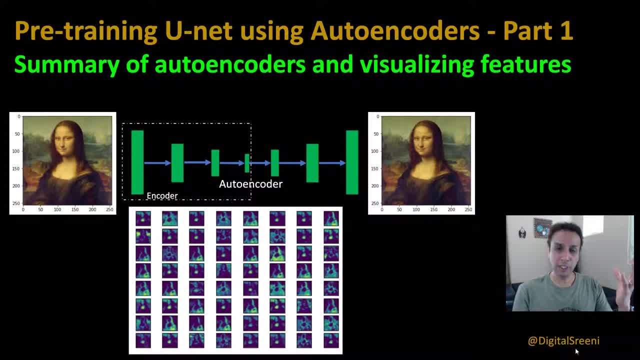 variables, right? I mean, in U-Net, you have your images and you have your masks and you're training on it. Well, that is exactly where auto-encoders come into picture. What is an auto-encoder? It learns how to reconstruct your image based on, you know, your input image. It. 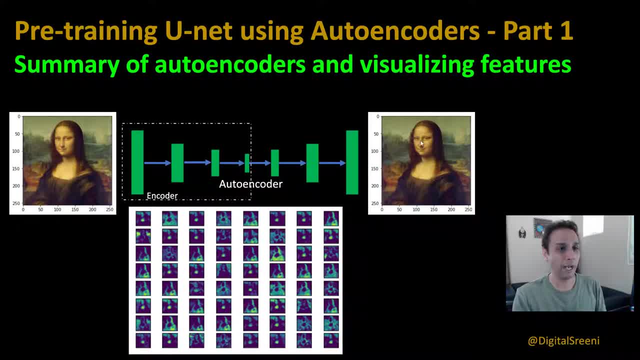 learns how to reconstruct your input image. In this example, you can see how you have a reconstructed image. This is an actual reconstructed image and not the same image. Okay, so you train this network where it goes From a larger size to an incrementally smaller. if that's a word, incrementally smaller, you know. 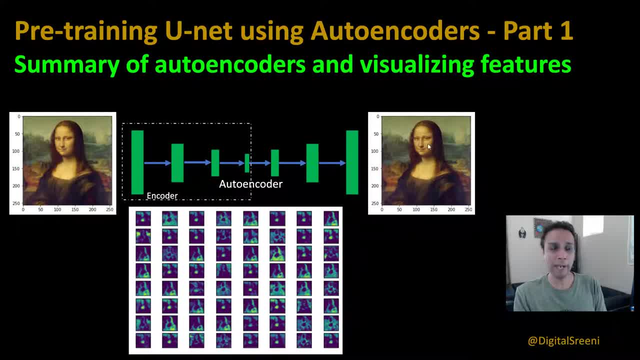 representation of your image and then you're decoding it back to original. In this process, when you're doing this, we are updating the weights of all of these and I'm proposing train that do that and take the weights from your encoder and use them as part of your U-Net, because U-Net is. 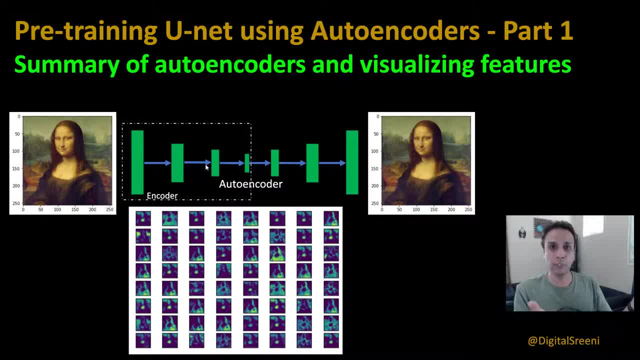 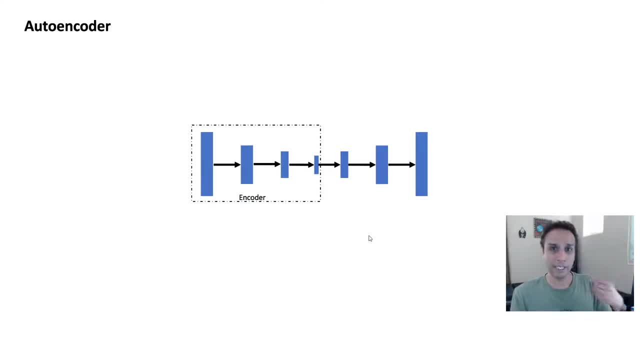 nothing but an encoder, decoder Network, just like auto-encoder. So let's get into the next level so we can understand this, and then we'll get into code in a minute. Okay, so I just explained that this is your encoder, right in a 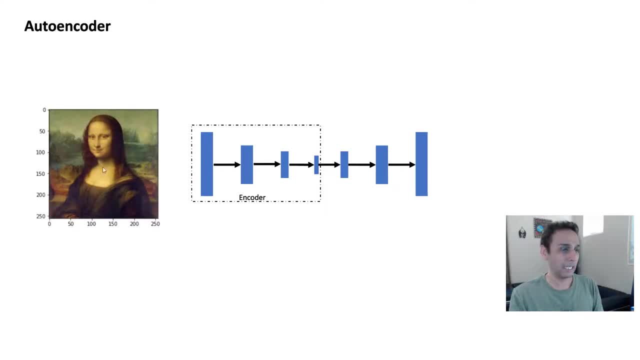 auto-encoder network. Now what happens, like when you send an image through it trains this network may take I don't know how many ever epochs and then at some point you're like, okay, let me send you an input image, and then it reconstructs that input image back right. So this is the different. 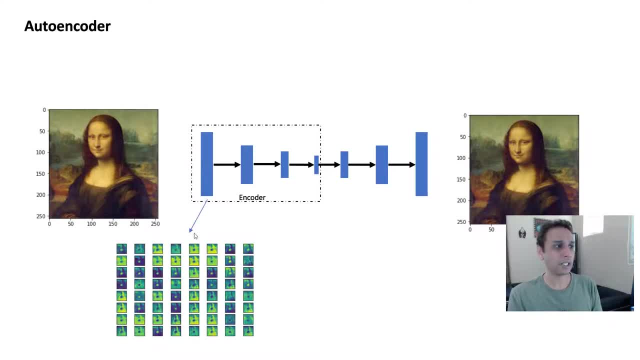 the definition of auto-encoder. During the training process it learns different features at different depths and it learns- I don't know- the edges are basic, you know. you see how there are certain edges going on right there in Mona Lisa and in some images. you can see that, And as you go, 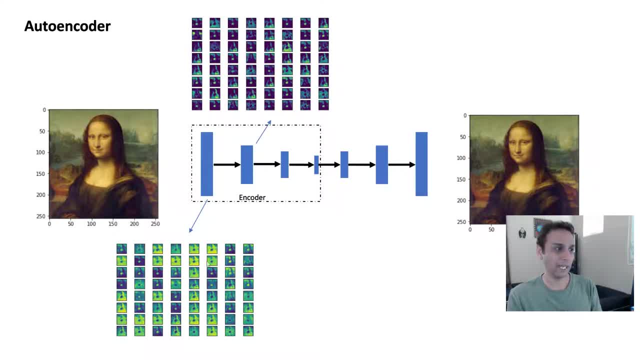 deeper and deeper, it's actually learning higher and higher features. In fact, the outer layer features may look the same between random initialized weights and pre-trained weights, but as you go deeper and deeper, it's actually learning higher and higher features. So this is where you 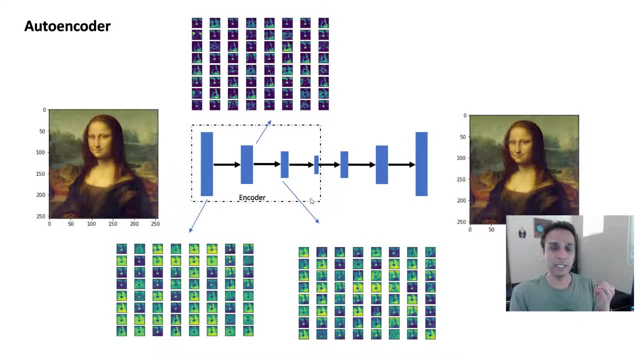 actually see some difference, because this is where the it's feature rich. now, Okay, at outer layers it has a very much knowledge of pixel awareness. let's say, as you go deeper and deeper, it's more feature rich. Okay, so that's why it's it's if we can pre train this and take these weights and use. 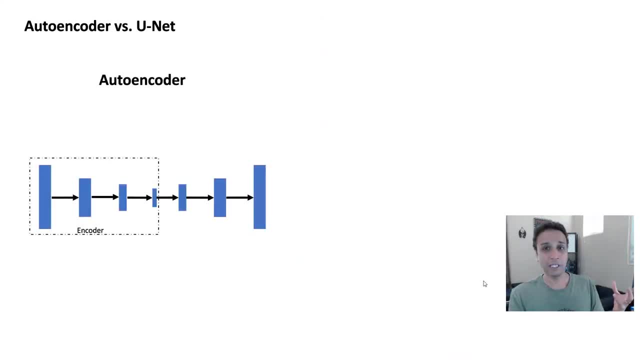 it as part of unit. that would be amazing. So let me just show you a few of these. you know, let's start with similarity between auto encoder and a unit, right? So if you look at auto encoder again, this is the third time we are seeing in this part of presentation. this first part is: 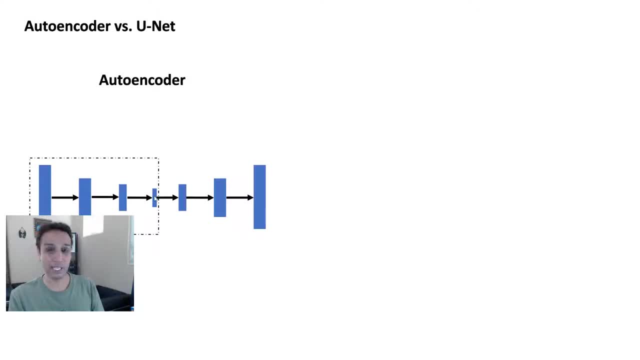 encoder, because we are encoding a larger size image into a smaller size And then we are decoding. this part is the decoder. So if you look at a unit- hopefully you watched my the last 30 videos or so where we have been talking about unit- So if you look at unit, this is exactly the same. 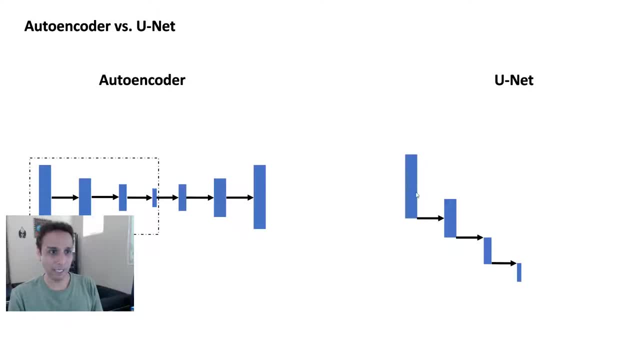 except you bend it into a U shape, So you have a encoder right there. right, This is nothing but this. Yeah, I just arranged it in such a way that it can form a U using this. that's it, And you have a decoder. So it's exactly this and that. Why is it called a unit? Because 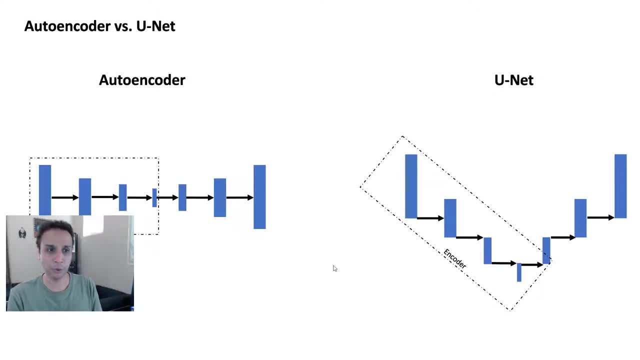 in addition to this, in addition to an actual auto encoder, we have skip connections, meaning the information from this layer is going to that layer and information from here is going to this layer. Why Remember the earlier layers? right here, they have information about pixels. As you go deeper, you have information about features. 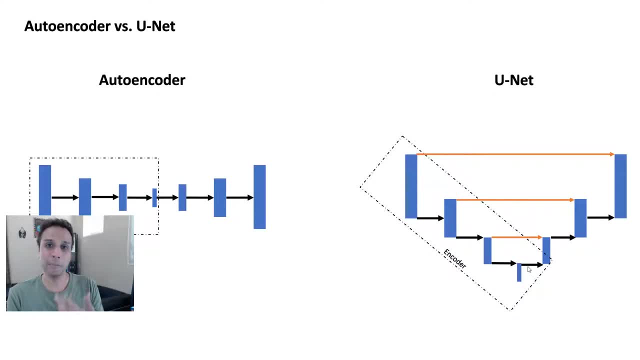 more information about features. A combination of this gives you semantic segmentation, pixel awareness plus the feature. Yeah, So that's what a unit is. This is exactly why I'm proposing to take if you have a million images that are completely unlabeled, if you have labeled data. 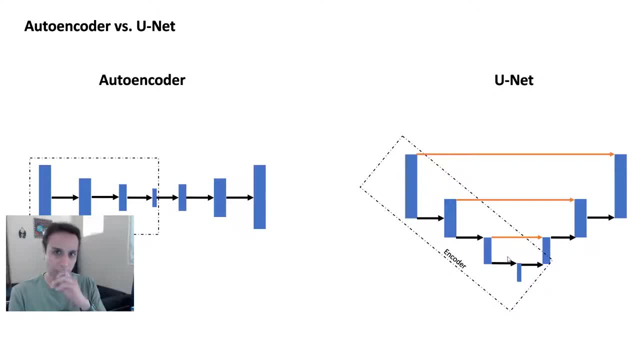 that's fine, Go ahead and train a unit and then you're okay, So you can just spend this. but then if you have 1 million unlabeled images, how can you benefit from them by not labeling every image? So just dump all those million images. train an auto encoder. 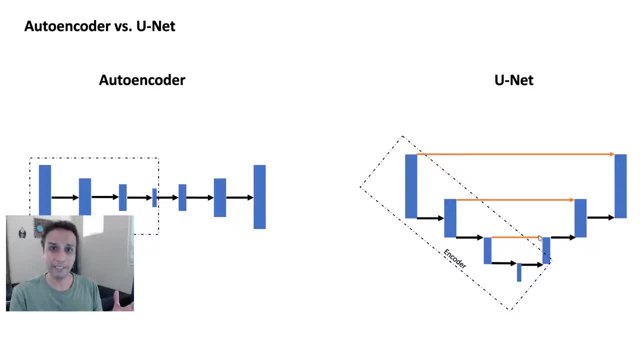 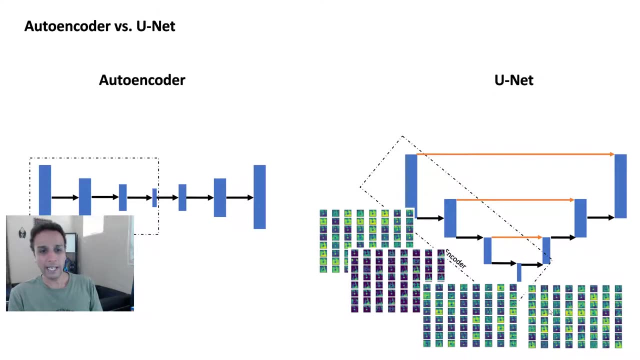 and then just get the encoder part and use it as part of your unit. This is exactly what I'm proposing right here. Okay, So again, information as you go deeper and deeper gets more feature rate. So let's just compare that with a few features. By the way, when we jump into the code, 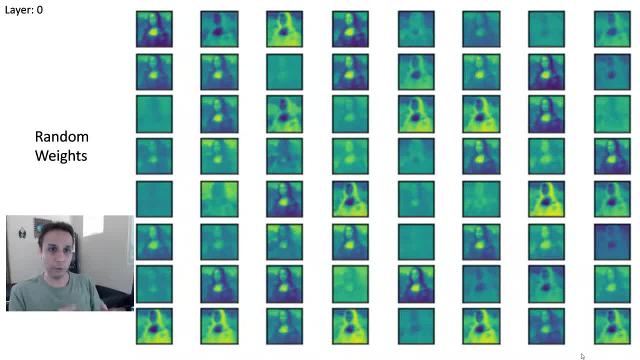 I'm going to show you a quick auto encoder And then how to print out these features at various depths of your network. Okay, So we'll get there in a second. So here is the feature output at layer number, the first layer. Okay, 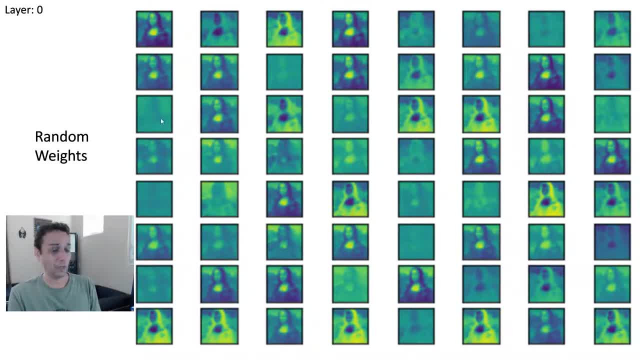 After the first layer- this is not the input- but after the first one, a convolutional layer. this is how your input looks. sorry, the features look like: Okay, So, as you can see- I mean you can still see Mona Lisa right there- So it's still trying to learn, even though these are random. 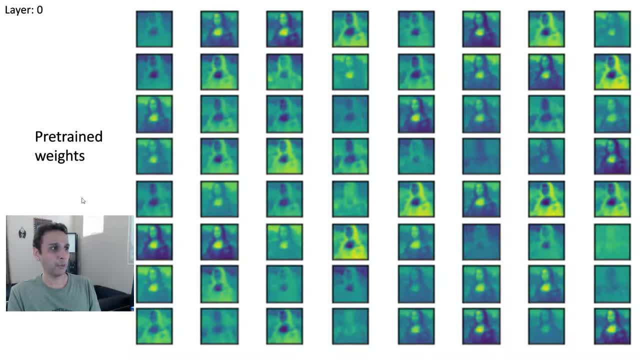 weights. but if you use a pre-trained network, this is how the weights would look like. It may not look that different but, again, if you try to squint your eyes, you can see the difference. where, in this case, where you have pre-trained weights, some of the features are, you know, 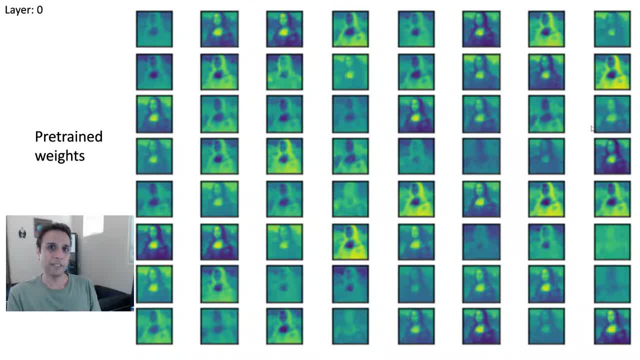 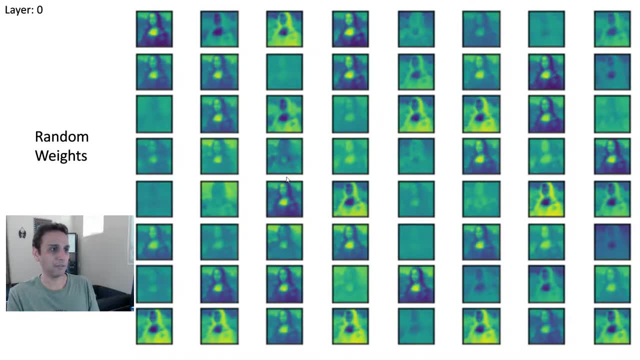 right there Some of the features. you see the hotspots right there. Yeah, You see hotspots. wherever you see hotspots, That means it's learning something, right there? Yeah, So that's the feature response right there. So there you go. 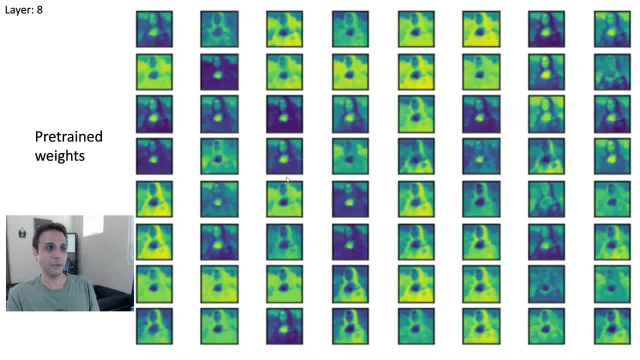 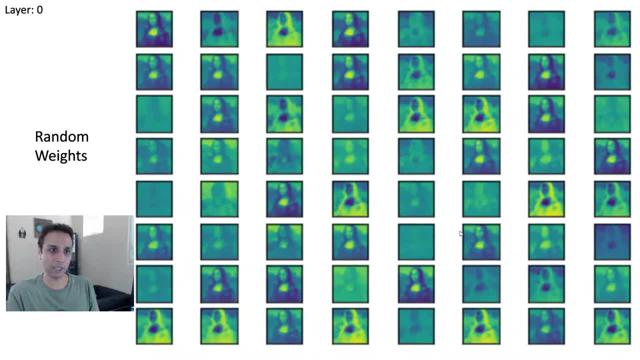 Let's go to layer number eight. Now you start to see the difference between random weights. Random weights still look pretty much the same as before, right, As the layer number one. let's go back. This is layer number zero. These are all random weights. This is pre-trained weights. 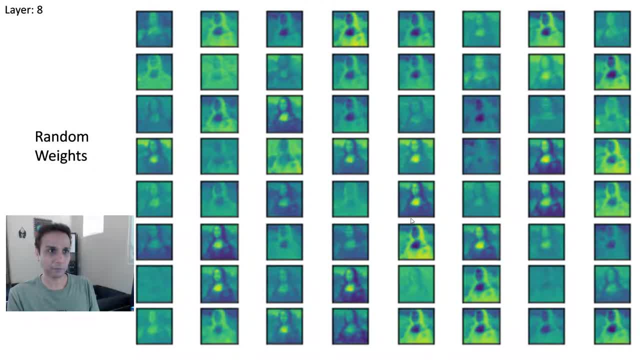 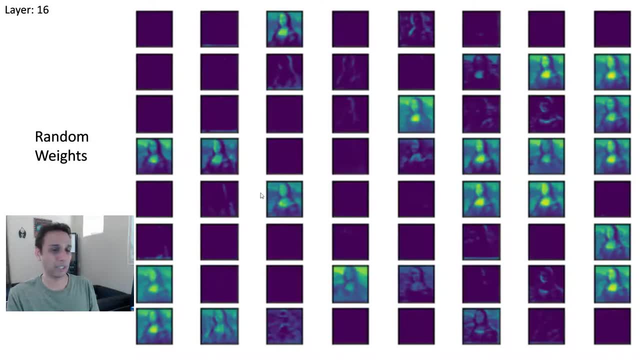 This is layer eight. Looks very similar to layer zero because these are random weights and this is pre-trained. Now you see much more definition of the structure. Now let's go to layer 16.. Again, these are random weights at layer 16.. 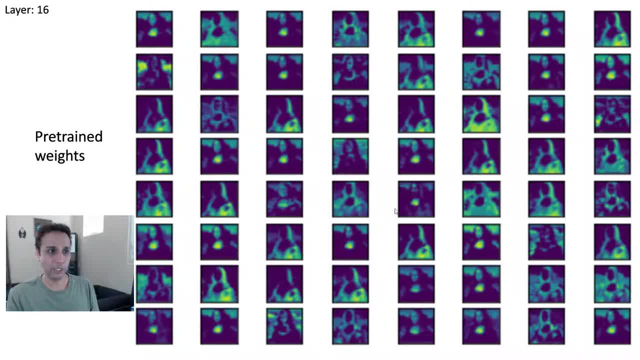 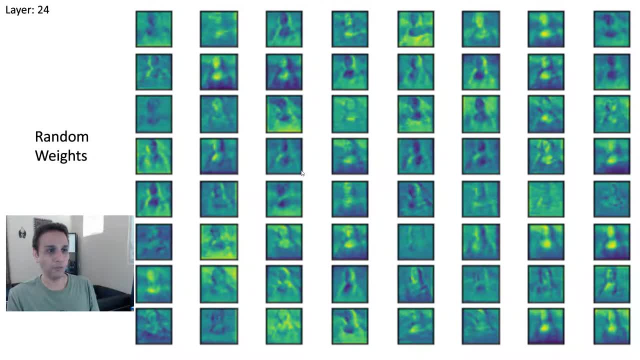 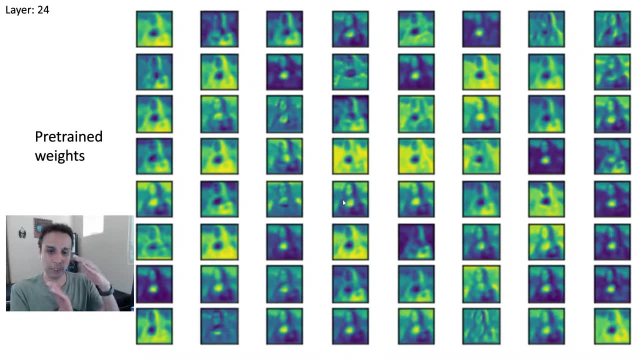 Okay, And this is pre-trained weights. You already have a lot of rich information. And finally, let's look at- well, let's look at a couple more, Layer 24.. Again, random weights, everything random, And here you start to see some structure. They look a bit more blurry because we 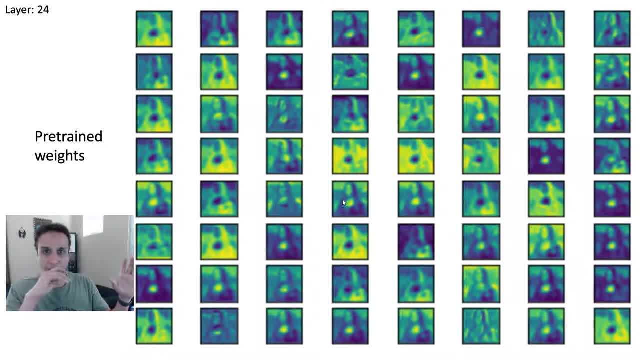 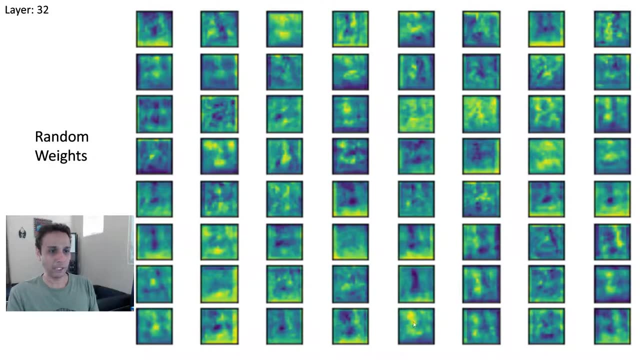 are going smaller in size and I'm expanding that. That's the only reason they look very blurry compared to initial. So, as you go, deeper features, feature rich, but not necessarily spatial. okay, So there you go. So, and finally, 32 layer. it's not like you don't even you see anything. 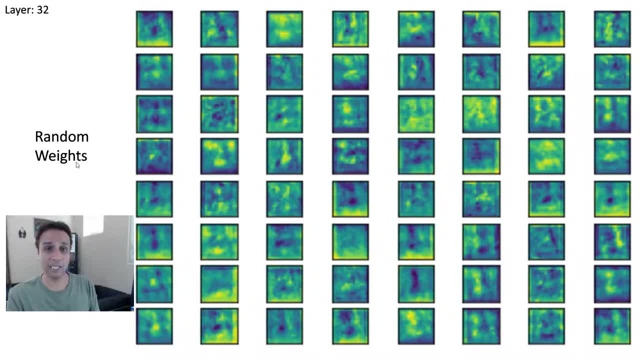 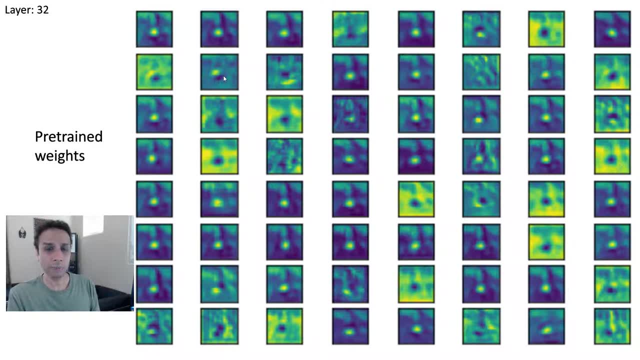 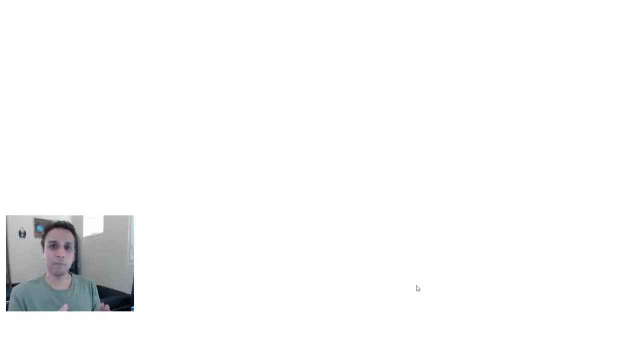 here You don't even see Mona Lisa anymore, because these are all random weights. again And again, with the pre-trained weights, you have hotspots showing something important, something useful for segmentation, for, for for reconstruction, right there. Okay, So this is, this is the thing that. 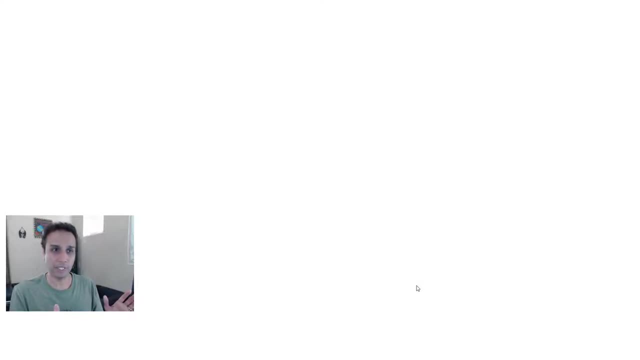 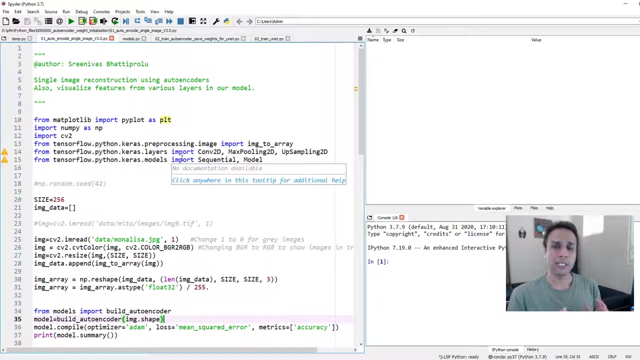 I wanted to convey in this video, like remind you what an auto encoder is and how to extract features. Jump into the code to repeat this, Okay, Okay. So let's start by understanding single image reconstruction in this video, just like what I've shown you in the presentation part, And then look: 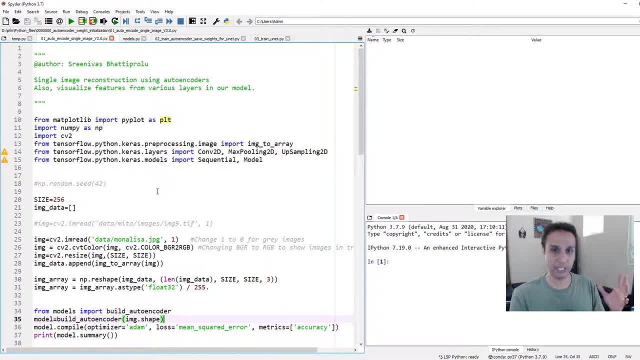 at some of the features. I'll share the code so you can do this yourself. This is a very educational thing to do If you want to get into auto encoders or even any any deep learning. this. this really helps you understand the features right at various various layers. Okay So, 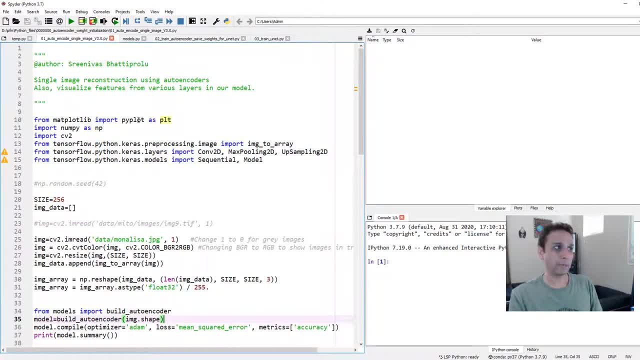 where do we start first? Let's go ahead and import the required libraries: matplotlib, numpy, OpenCV. Let's go ahead and do that. This is actually. first. let's make sure we are in the right working directory. So, again, I'm using Python 3.7 and TensorFlow 2.4.. So let's look. 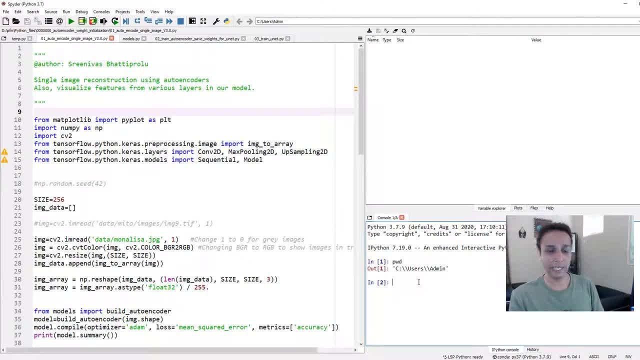 at my present working directory. That's definitely not where I want to be. I can navigate through here or I'll just type some mistake right there And it says: Hey, this is not a good code. You know this is a mistake, So let's now. if I do my directory, it changes. 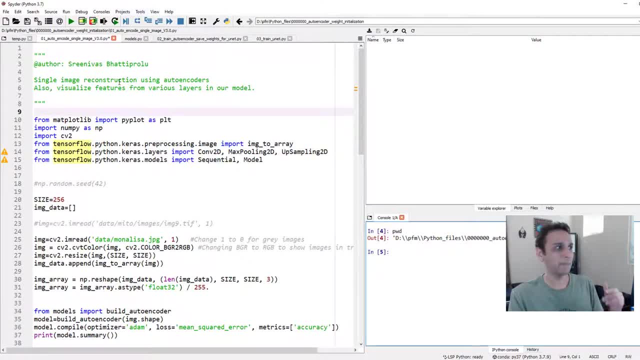 because the settings, the way I have settings in my spider, uh, anytime I run a run a file, it just automatically changes the working directory to that. So this is the easiest way. Anyway, little tricks. Now let's uh run these lines of code: And uh, let's also from: uh, 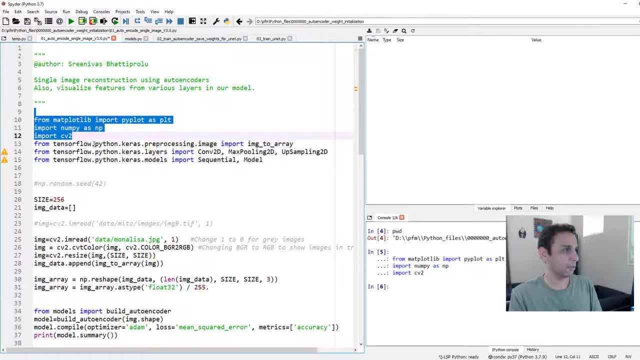 from Keras? uh, I'm going to. why did I do TensorFlow dot Python dot Keras? Uh, sorry, I am supposed to edit the code while I'm doing a video, because I have no clue how that's going to work out. Normally I just do: from Keras dot reprocessing: import this. from Keras dot layers: import this. 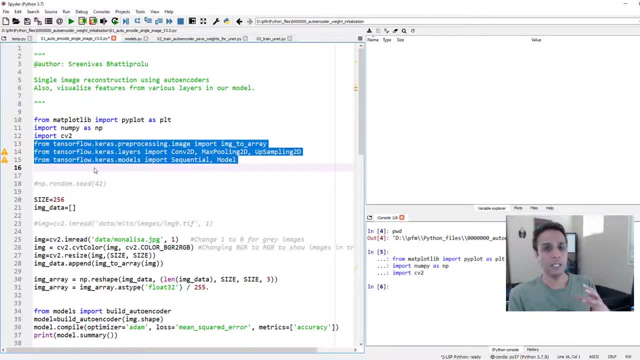 but uh, uh, but uh, since I switched to, uh, Python two point something. uh sorry, TensorFlow two point, I started to do TensorFlow dot Keras. Okay, Just my personal preference. Uh, otherwise I used to directly import Keras previously. Uh, 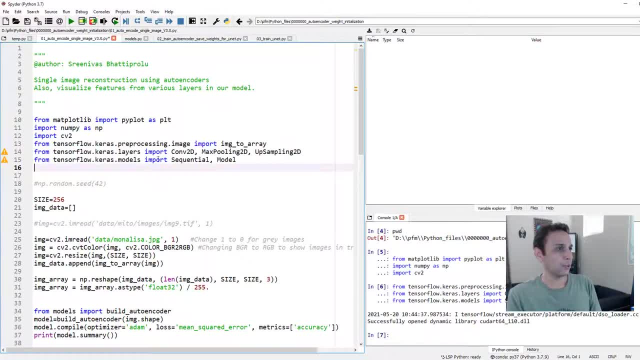 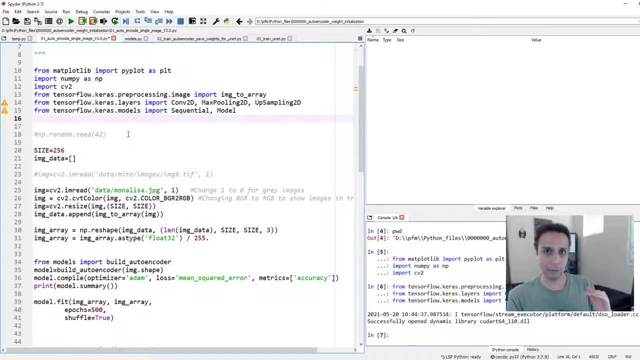 just just a habit. Okay, So there you go. So, uh, again, I don't think we need these, but this is something that I usually import if I'm trying to build a deep learning model. Okay, We'll. 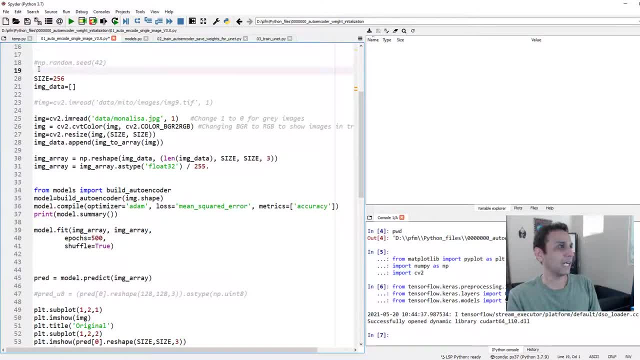 we'll go through these step by step in a second. This is pretty straightforward. I want to resize my image to two, 56. So I just defined it here. and my image data, which I'm going to capture. uh, am I going to capture image data? I don't even, I think. yeah, right there, image data. 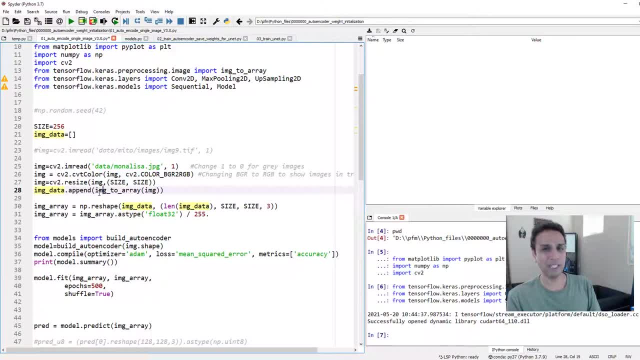 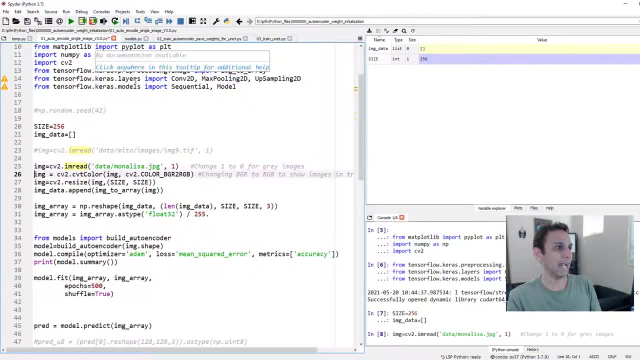 empty list because I want to append my image into array. This can be useful if you have multiple images, right? So, anyway, let's go ahead and define this, and I'm going to read my Mona Lisa image right there as color. 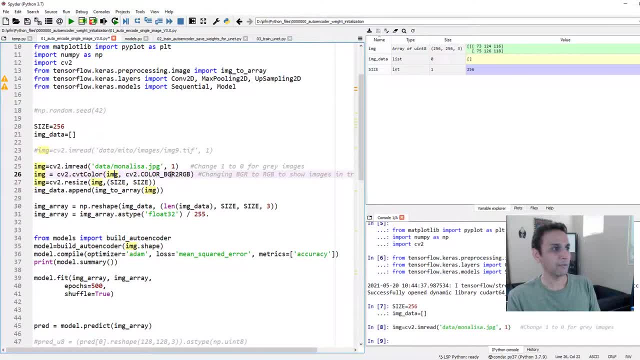 Yeah, All channels and convert my color from BGR to RGB. That's not a necessary step, but I do that usually if I want to visualize things, So that makes it easy for us to intuitively understand what's going on. Okay, Now I'm going to resize my image. I think this is probably two, 56 to begin. 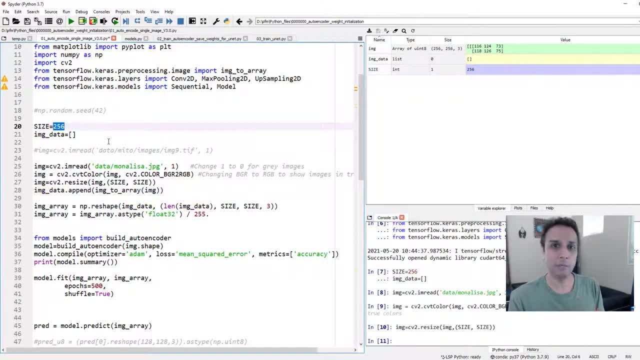 with. but uh, that's okay. I mean I'm, why am I resizing? Because my network expects two 56.. That's pretty much it. Okay, Now let's go ahead and image data dot append And finally reshape this area. Why am I doing all? 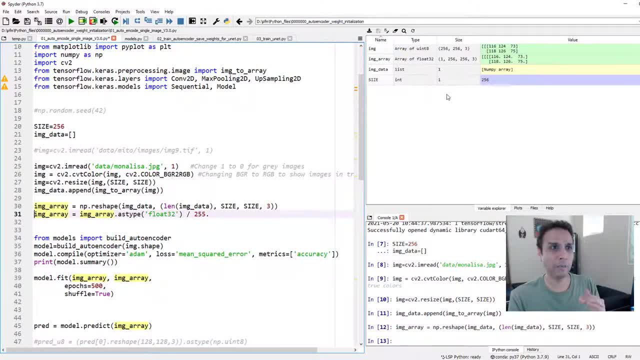 of this Because, uh, for the network, I want my input to be in the shape of N, X, Y and number of channels, right, And his number of images: X, Y, image dimensions and number of channels. This is obviously, uh, you, you probably. 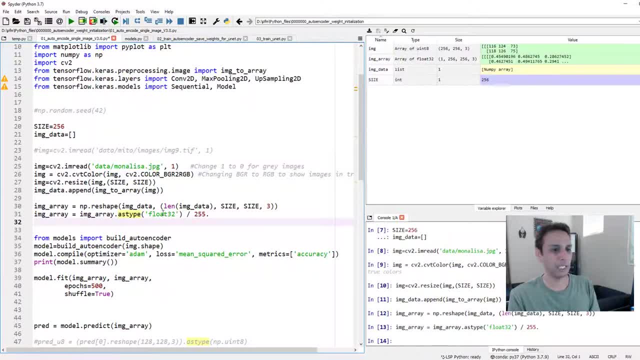 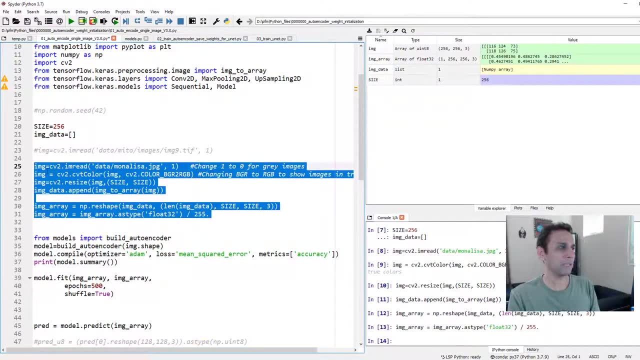 you know that. anyway, let's go ahead and divide the pixels by two: 55.. So it's a, it's a way of scaling. So now I'm already. my image area is, uh, float 32.. So up to this point, I should probably. 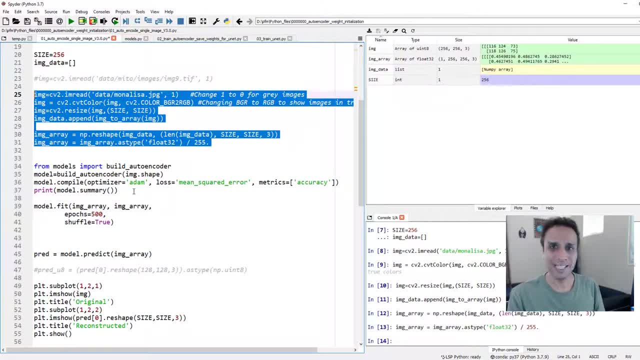 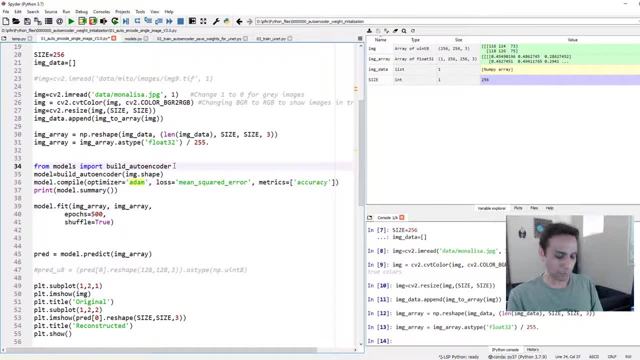 have skipped through this and just said I'm loading an image, That's it Right. But again, my viewers come with various backgrounds, So this, hopefully, can help. Okay, So now comes to the auto encoder part. So the what is the plan now? we have an image we need to encode and we need to decode. 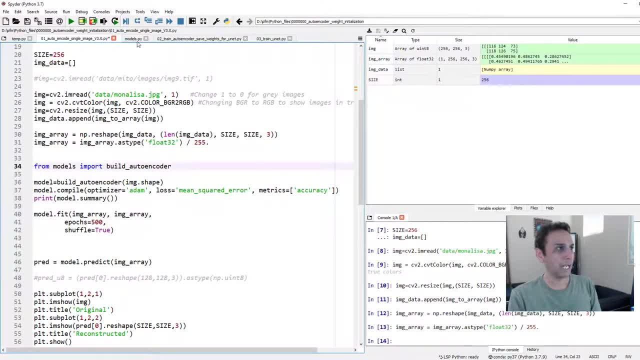 this image: Okay. So I Okay build a model. I mean, I have a file called models uh, where I have a uh function to build auto encoder. Let's go through that now. Okay, So I'll share this again with you, This one, what I have. 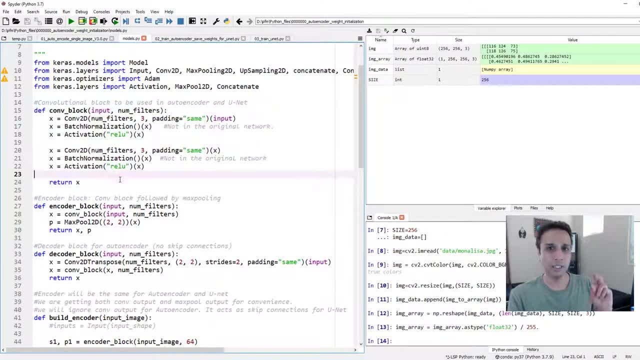 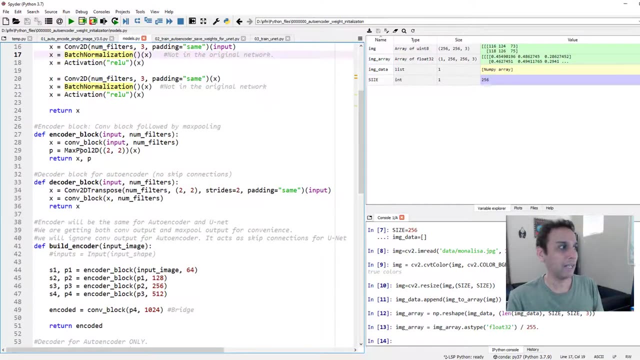 defined is, uh, a convolutional block, a function that that builds a convolutional block that has con, two convolutional layers, And, of course, activation for each of these layers and batch normalization. So this is a convolutional block. And then I have it: Encoder block. What an encoder block is basically a convolution block. 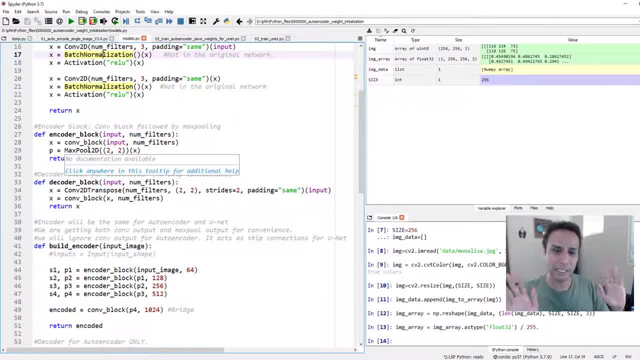 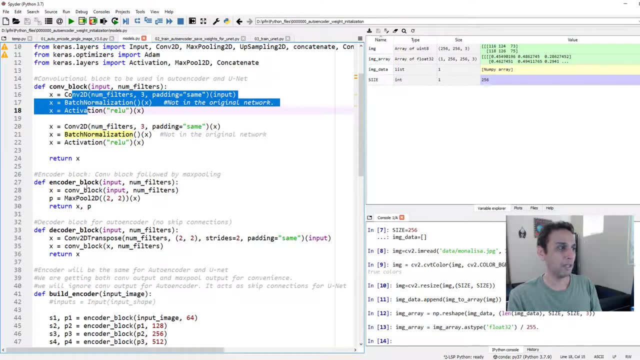 plus a pooling layer. That's it. This is again nothing new unit. We have built a unit this way. Okay, So a unit is basically a convolutional block plus max pooling, Right? So and then you keep going and then you do the decoder block. Okay, So, so far, I hope makes sense. 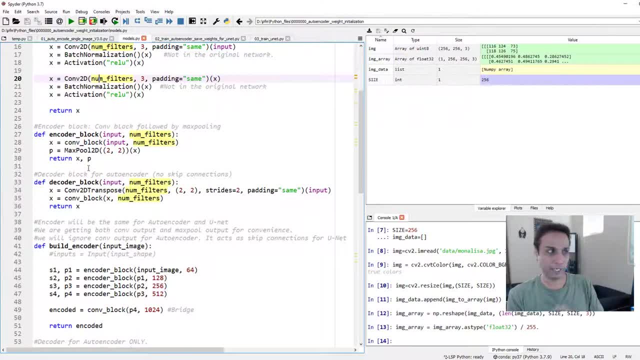 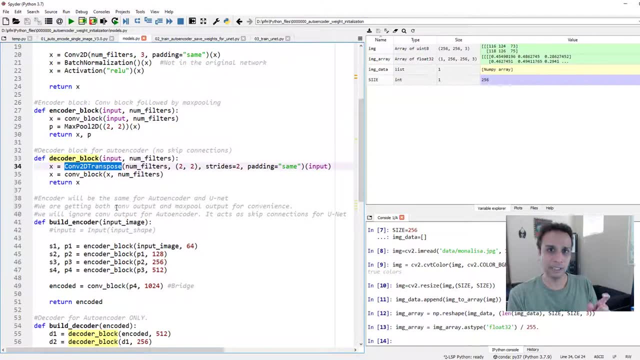 This is my encoder block, A block of, uh, you know to build my encoder, the decoder block is, uh, Exactly opposite. instead of convolution, I have transposed convolution. Yeah, to go the other way. think of this as upscaling. 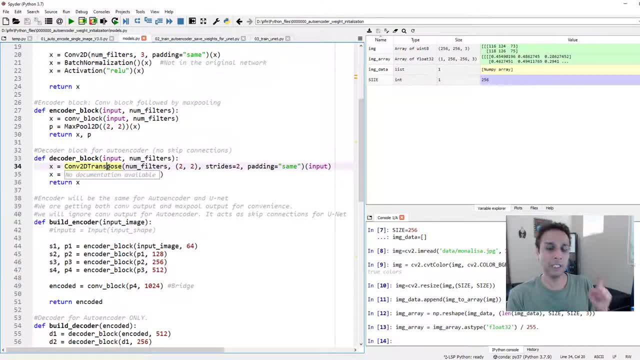 I have made a video on this topic: difference between upscaling and con 2d transpose. Please watch that video if you don't know what the difference is between these two. But either way, in the decoder part we are going to use along the decoder path, We are going to use con 2d and the convolutional block. Okay, This is again our decoder side. 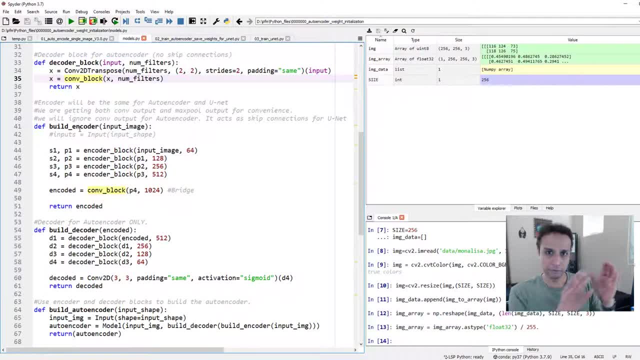 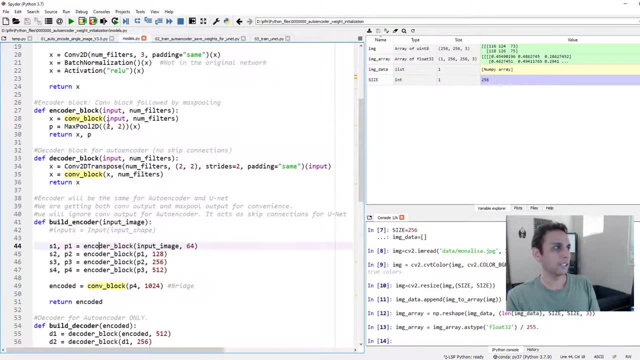 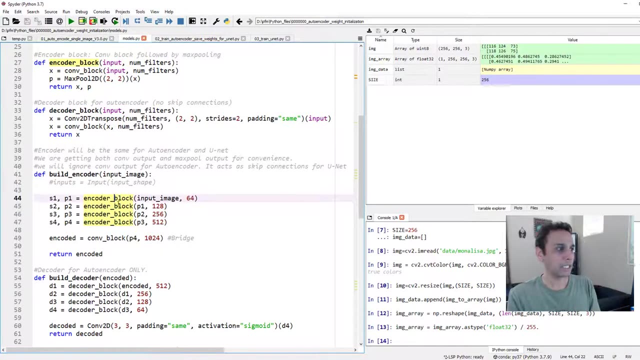 So let's go ahead and build our encoder. Build our encoder, Yeah, going from a large image to the smaller. How do you do that? my encoder block. Right there We have my encoder block. I'm repeating that four times. It's up to you how deep you want to build. the reason I built it this way is I would like to use exactly the same. 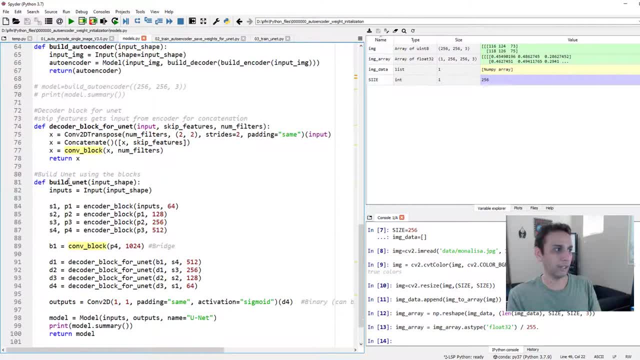 Encoder when I build my unit. later on, when I build my unit, I would use exactly the same structure. This is why I can use the weight From there to here. okay, that's the whole goal here. Okay, so I'm going to build my encoder using four of these and progressively. 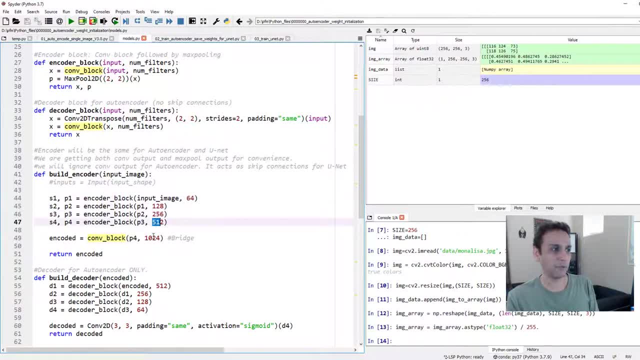 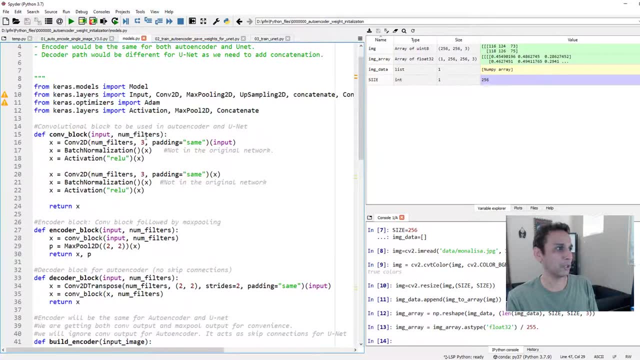 I'm increasing the number of filters from 64 to 128, to 56, 512 and 1024 and Progressively your image gets smaller as you go. Why does your image get smaller? because in our convolutional block you have 3x3. 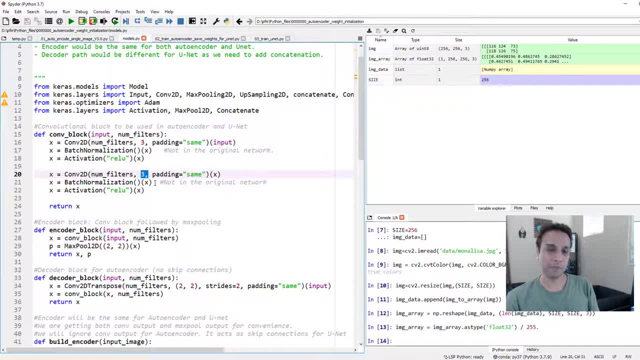 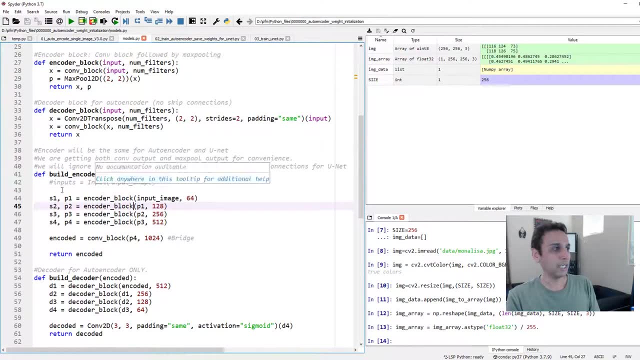 Kernel that kind of brings your image Smaller and smaller as you go through these layers. I hope you you know the basics of that right. so That's building the encoder. and what does the encoder give out as outputs? We are actually getting two things as outputs. 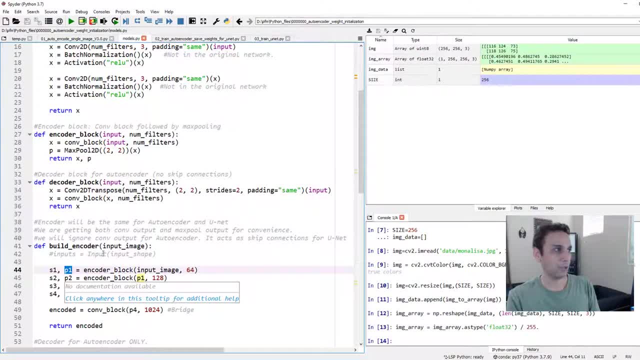 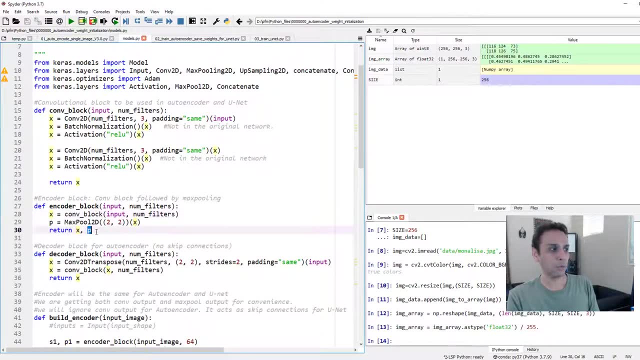 For auto encoder. we are not going to use both, We are just going to use one output. But what is my encoder block giving out? It's actually giving out the output of convolution block and also the output after the pooling. That's it. The whole point of encoder block is to make sure we get two outputs. one is an output of just the convolution block and the output. 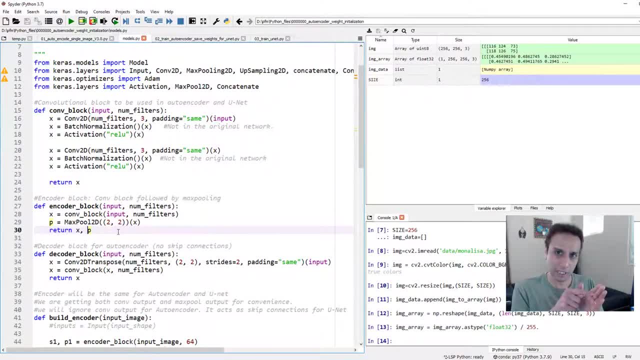 after max pooling. Why? because in unit- remember the skip connection part, The X, the output of convolution block, is what's being added to the next level in the decoder. Okay, Again these. I assume you know these basics. Otherwise, this, this video, can be one of the most confusing videos that you have ever watched on my channel. 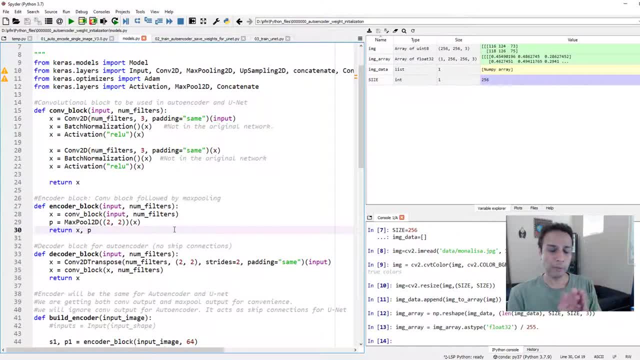 So so far, we are trying to build an auto encoder, and you may be thinking: why are you complicating things? Auto encoder is easy. Just put like ten lines of model dot. add, model dot. add, Yes, Yes, You will be right. But the whole point of this video is to show how the same encoder that I'm going to build 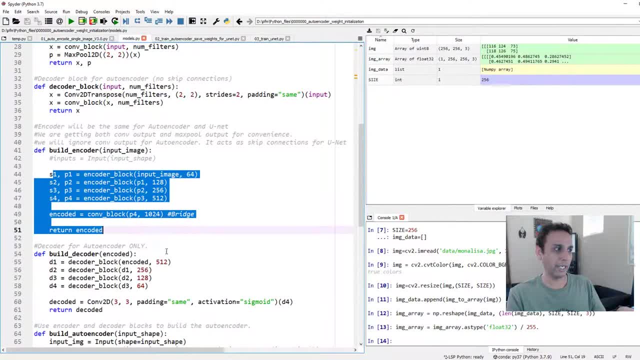 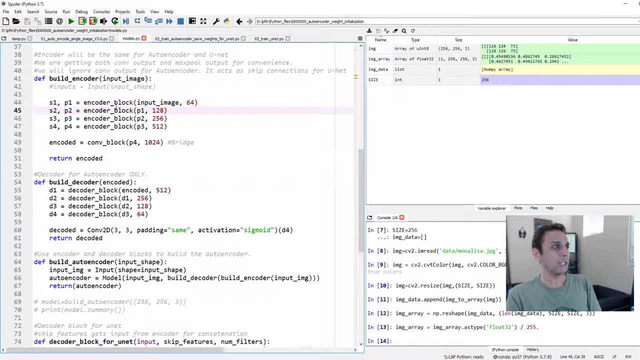 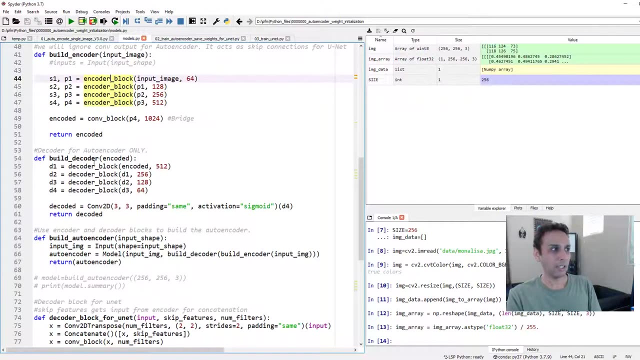 Is going to be used also in unit. So once we train this encoder and get the weights, those weights can be transferred to the unit. Okay, that's, that's our goal. so now you know how to build encoder: just These five blocks, and then My decoder goes from this point and then, symmetrically, goes the other way, right? 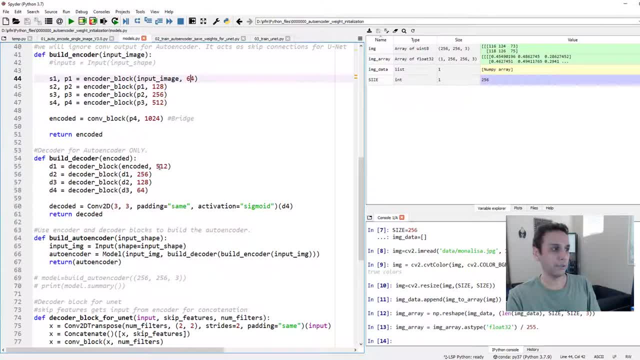 So ten, twenty four, and then five, 12, 256, 128 and 64. that's exactly what I'm doing right there, going the other way, and then finally it gives me a decoded image of whatever the input is, with three channel output: 256 by 256 by three, right? so that's exactly what we 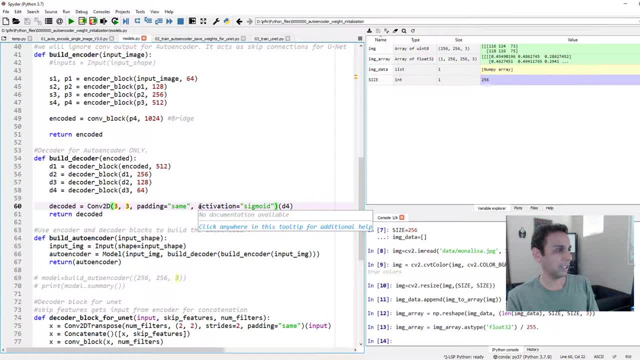 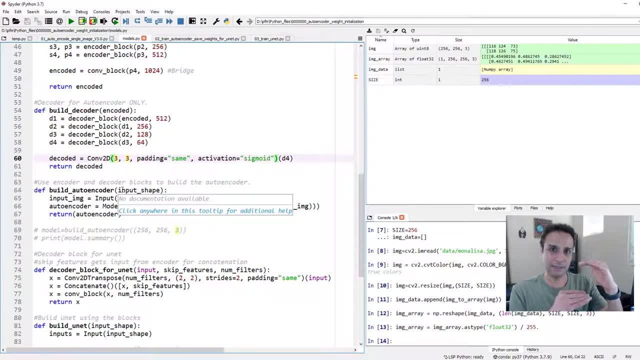 are doing and anything, anything. I think that's that should be it. and when we build an auto encoder, it's basically encoder plus decoder. that's it right. that's that's our auto encoder. that's exactly what I'm doing. my input is going to be my input image with a shape of that, and my auto encoder model is: 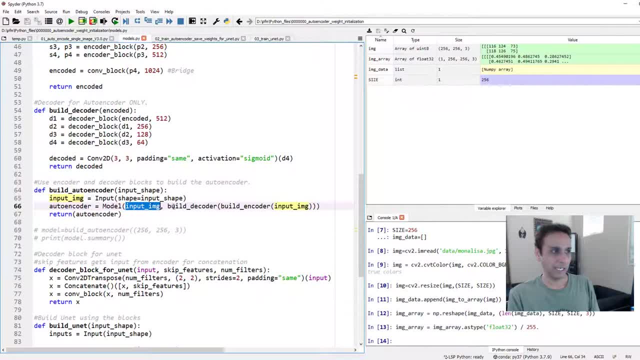 basically my input and then this is my output. right? how do you define a model, your input and output? input is my input image. what is your output? your output is basically that, a decoded image- and how do I define that here- which is nothing but build decoder, build decoder and input to the decoder is my 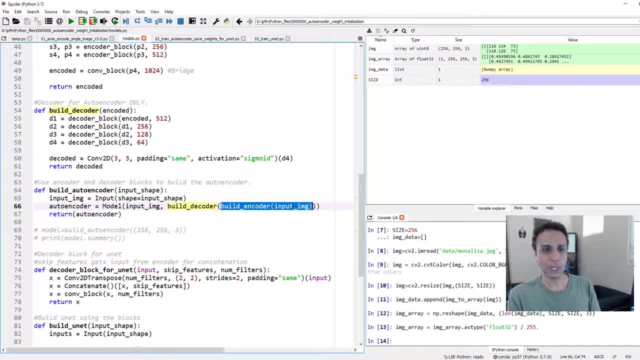 energy decoder encoded image, which is basically that. I hope this makes sense Again. some people may think this is too basic. Some of you may think, hey, what are you talking about? But watch this video a couple of times, practice this and things will make sense. This is a great, great way of learning. 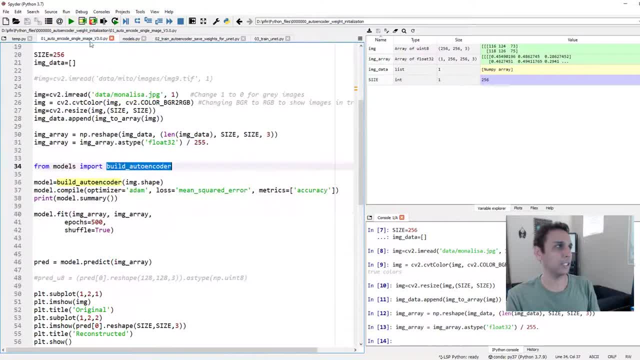 about. you know these neural networks. Okay, so much about discussing the model. Let's just go ahead and import our build autoencoder, the function that we just defined, that builds the autoencoder. What does the build autoencoder need? It requires the shape of my image, And what? 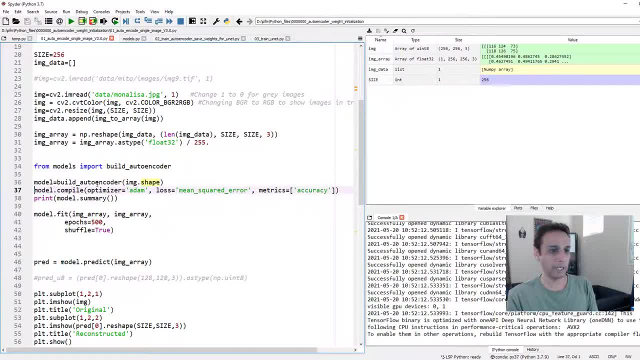 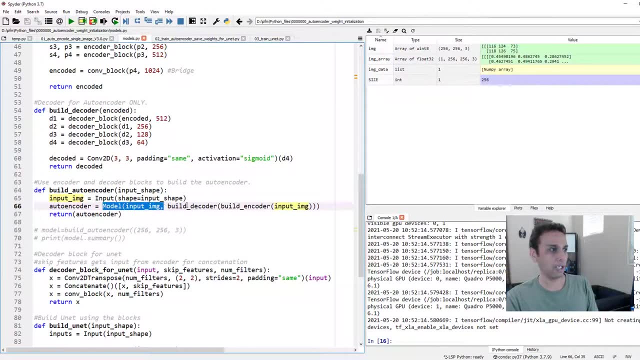 is the shape 256 by 256 by 3.. So let's go ahead and build this autoencoder. So it's building it right now. Basically, when I say build autoencoder, it's putting together this model with input image size as input, input image as the input and then the decoded as the output. That's exactly what it. 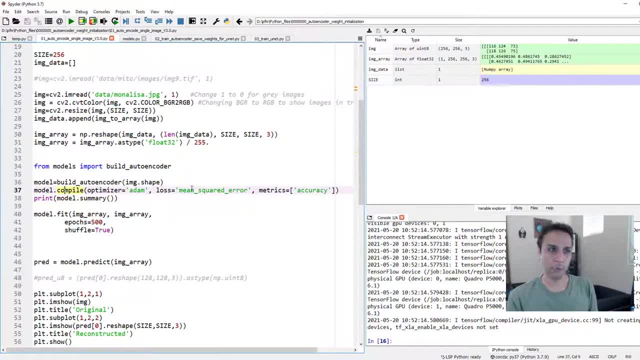 did. Now let's go ahead and compile the model. How do you compile an autoencoder? Well, let's use an optimizer called Atom. This works in most scenarios, And for loss, let's use mean squared error. Why This is not a? 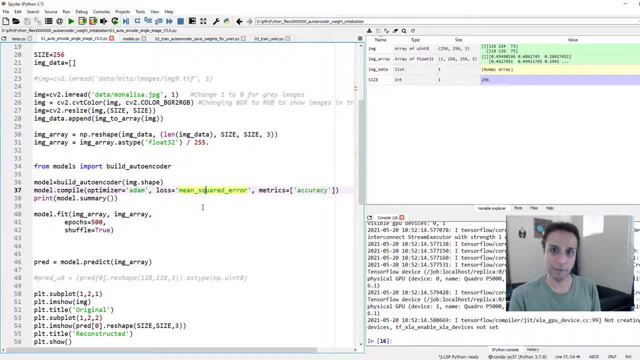 regression problem. Why are we using mean squared error? Well, in a way, this is a regression problem because we are trying to minimize the error between the output and the input images. right, We are trying to minimize this reconstruction error between the output and input. And if there is no, 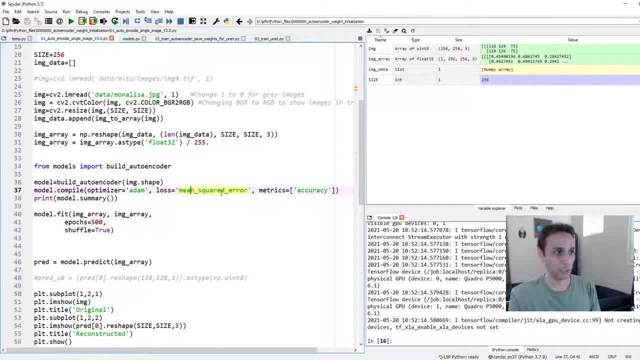 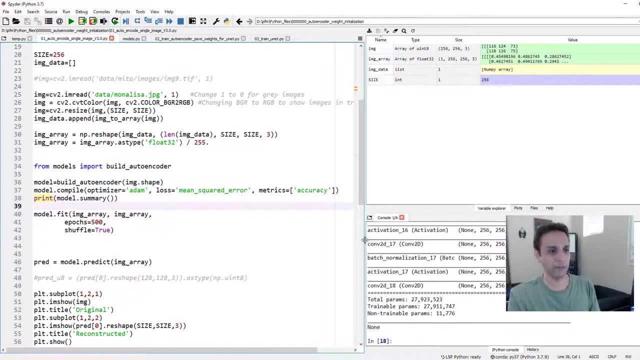 error, I get the same output as the same input. That's why I'm using mean squared error And we can track the matrix accuracy. So let's go ahead and do that And build that, And now let's print the model summary. This is basically my encoder: decoder. 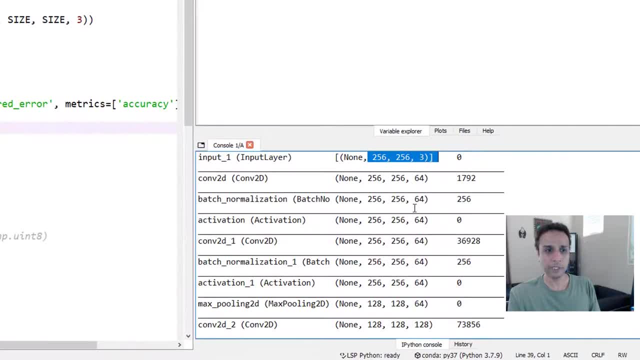 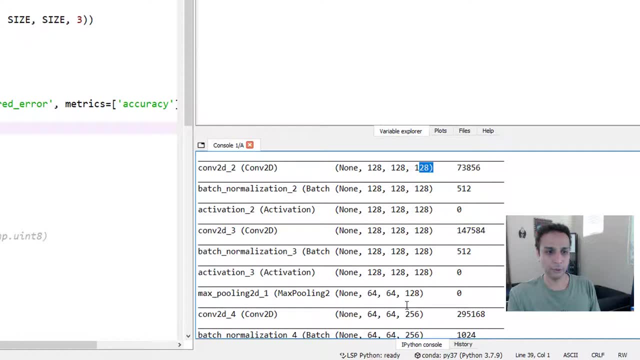 network. So I start with 256 to 56.3.. And then increase the number of filters to 64.. As you know, we did that 64 to 128,, 128 to 256.. So the filters increase. the size goes down by half each time. 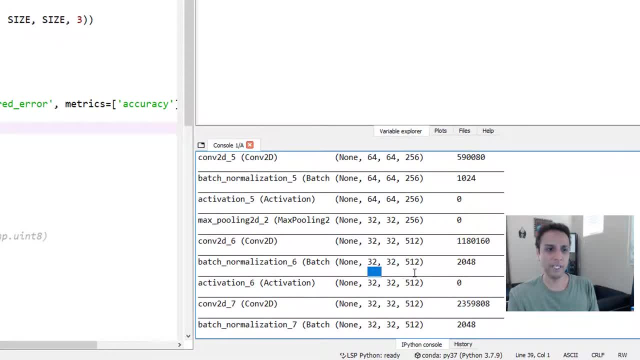 Yeah, the filters go up by two times. Okay, I think 1616 to 1024 is the last one, And then it goes up typically 32, 32, 512, 64, 64. And finally we'll end up with 256 to 56.3 image, And there are about. 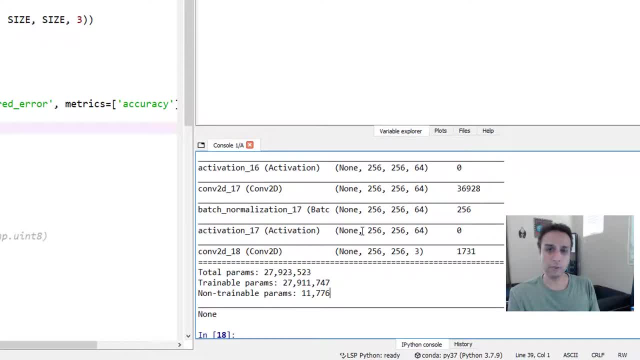 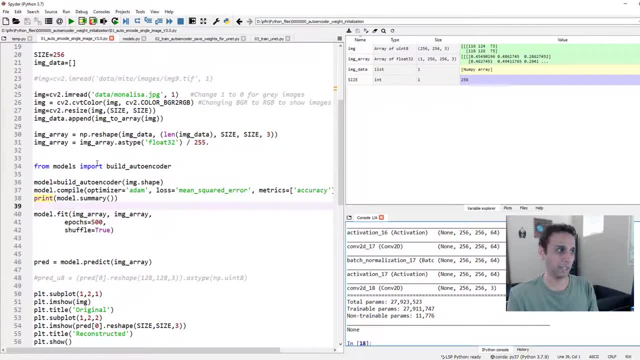 28 million parameters that need to be trained. But don't worry, this is just single image, So it's going to be super fast when we train it, because there's not much data, even though there are 28 million parameters that need to be adjusted. But I really want to make sure you understand this. 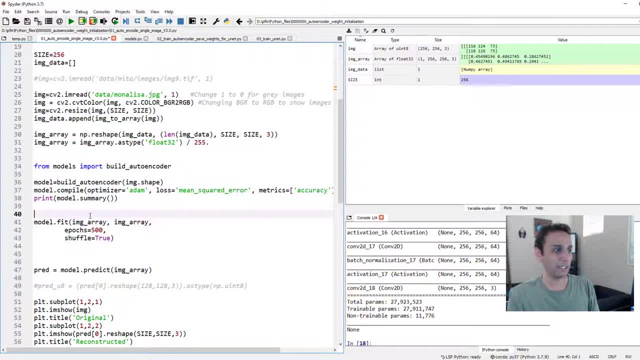 you know what we are trying to do, And let's go ahead and modelfit. My input is image array. my output is image array. Normally you give x and y. In my case, x equals to y because this is an auto encoder. we are encoding, decoding, Okay. 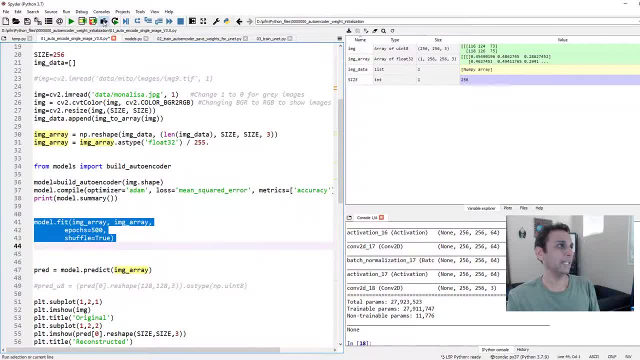 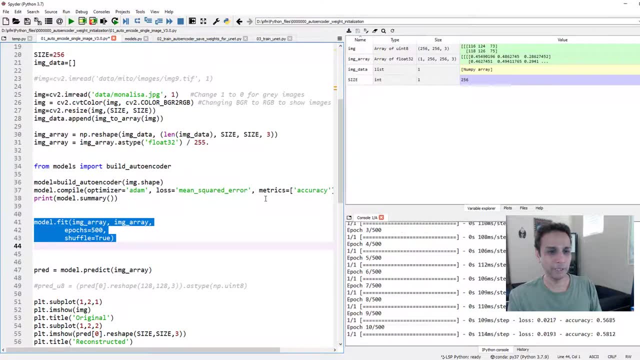 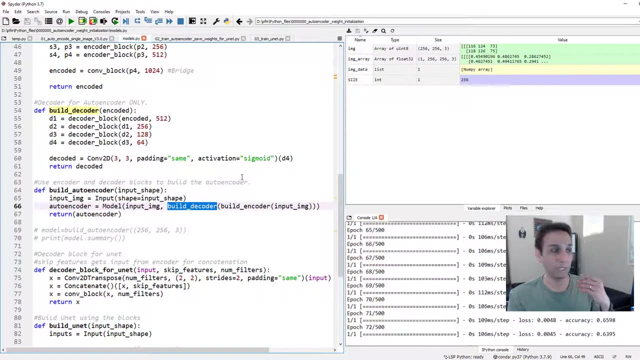 And let's run this for 500 epochs And while it's running, it should be pretty fast actually, Especially if you have a GPU. Yeah, there you go. It should be done in a minute or so, But just want to confirm one final time, but I just want to reinforce this message one final time. 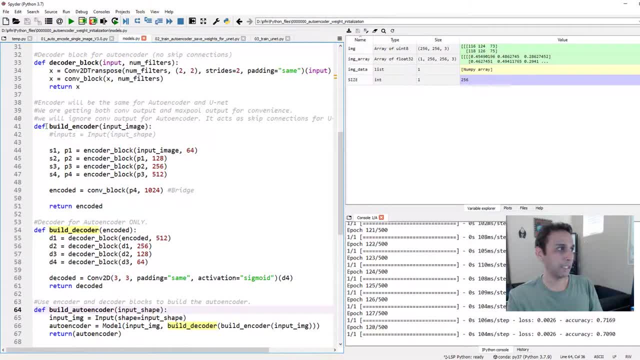 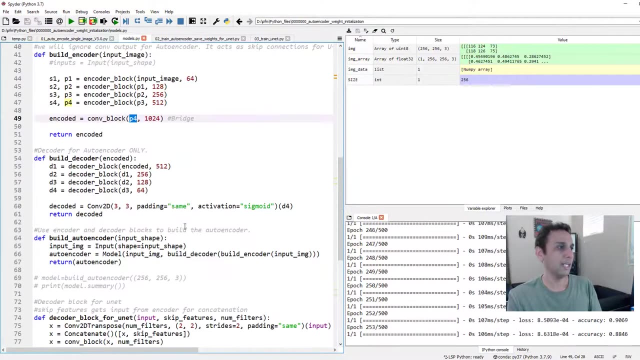 What we're doing is an auto encoder, where we did build an encoder that goes from some size to smaller size incrementally, because we have this max pooling- Sorry Yeah, These max pooling operations right there, the convolution and max pooling operations, and then the number of filters are going up incrementally. Exactly opposite is. 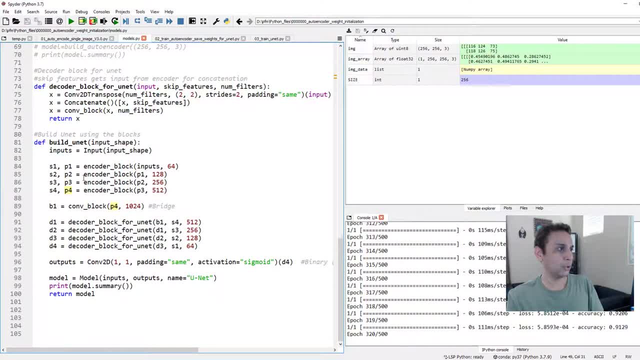 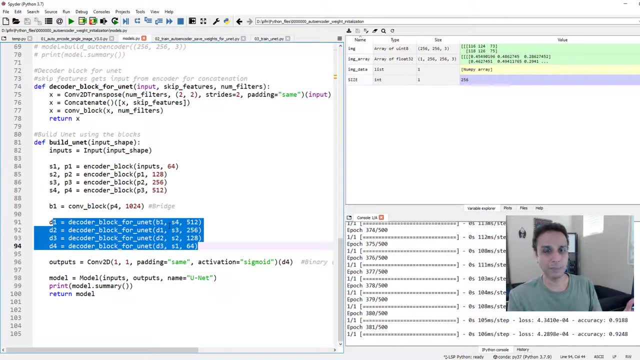 happening in decoder. So, as you can imagine, when I get down to unet I'm using the same encoder but then a different decoder. Yeah, If you just use the same decoder then it's auto encoder decoder Decoder block for unit decoder block for unit. needs the skip features. 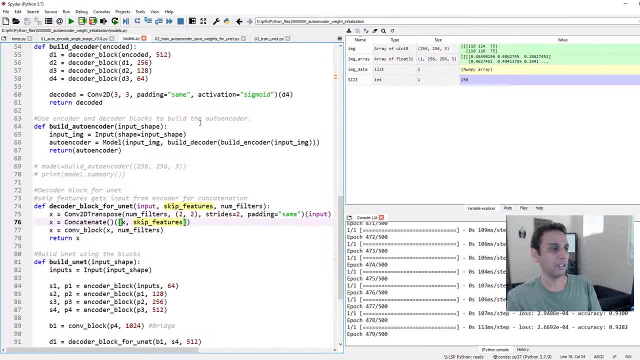 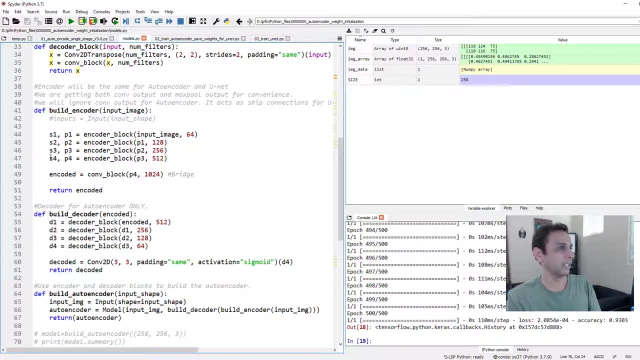 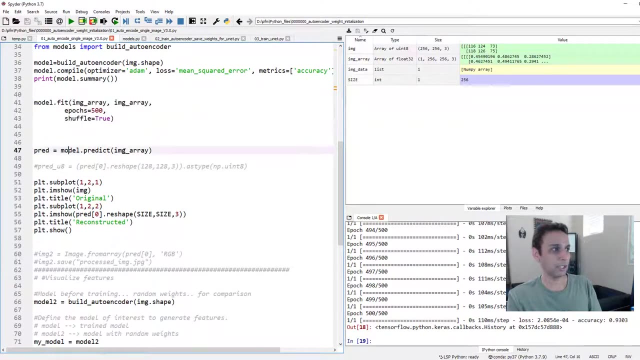 And we already know where the skip features are coming from. these are the skip features that that we get from here. Where is it? Where is it? Yeah, So these are the features. okay, there you go. the training is done, So let's go ahead and reconstruct, like predict, on the model you know, on my, on my original image. 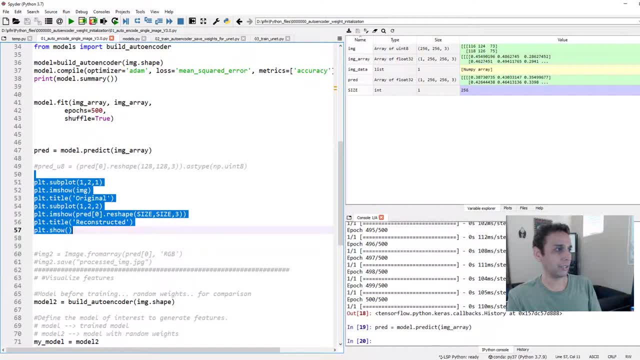 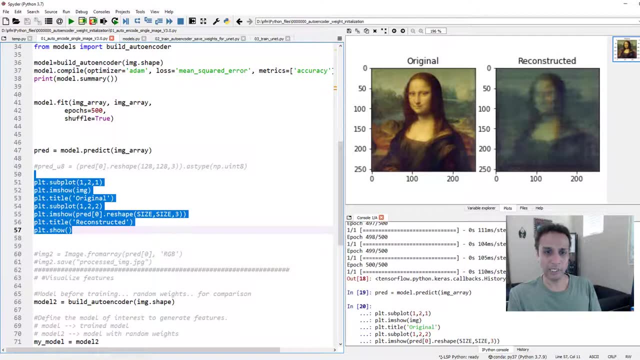 So hopefully it should reconstruct a decent image. so let's go ahead and print out the original and the reconstructed image. That's not. that's not a good reconstruction. so what kind of accuracy? 93, right? So let's do this. if you move one more time and I'll pause the videos. 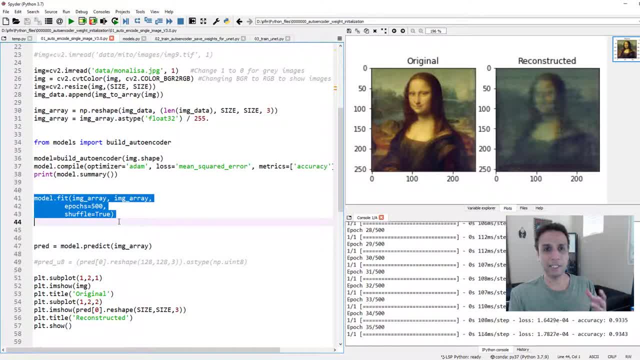 I won't waste your time and I'll pause the video, and then let's let's see How dramatically it comes. I remember if I did this like 1000 epochs or something, then then the accuracy was super amazing. Okay, so let me pause this and then continue with him- literally a few seconds, and 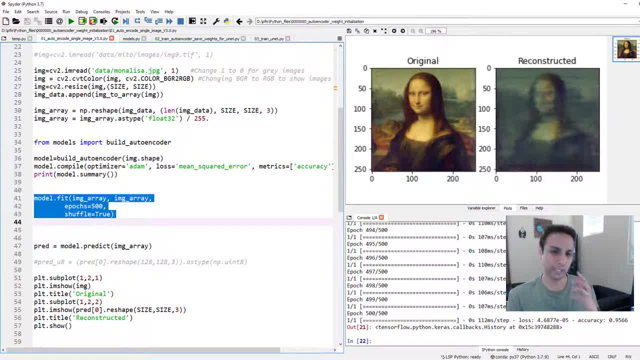 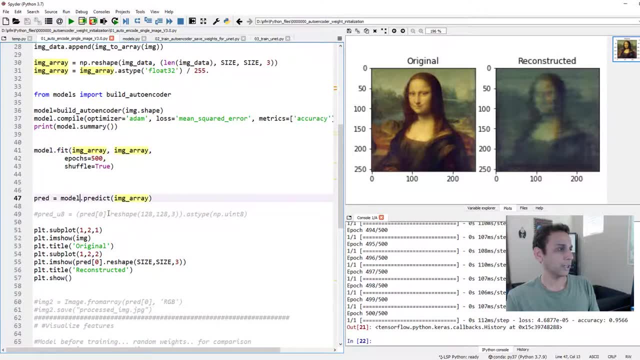 Yeah, a few seconds later now, We had about 93% accuracy. now This is about 96%, and let's see if it made any any difference. so what do we need to do? let's go ahead and predict this one more time using the new model, and 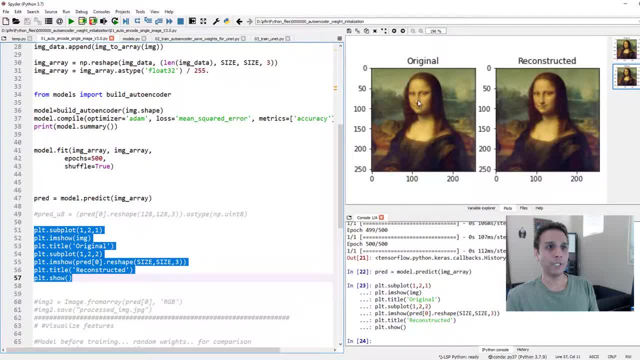 Let's print this again. Oh, there you go. right, so this is with 500 epochs, This is how the reconstruction is, and 500 epochs: this is where we got almost identical. I mean, I can see some difference in color. This is three channel image, right, but then look, look how good this is. this is a bit blurred compared to this one. 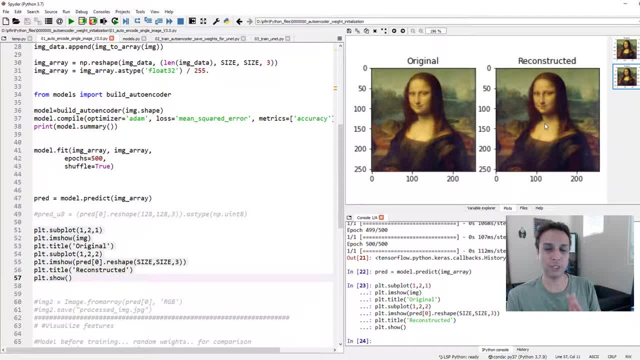 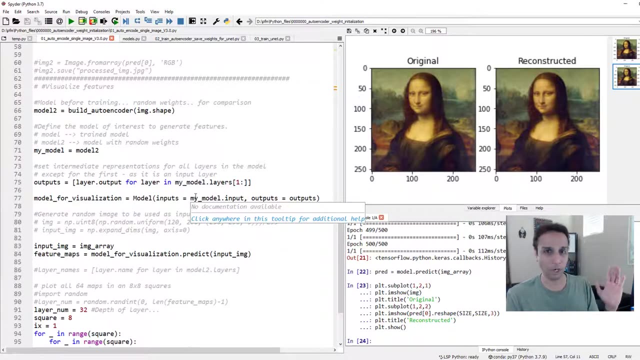 But amazing. but our goal is not to reconstruct the best image, our goal is to make sure we reconstruct it as good as possible. But then take the weights from the encoder, so just to show you that part, not not how to take the weights. I'll save that for the next video because I don't want to make this a one hour long video. 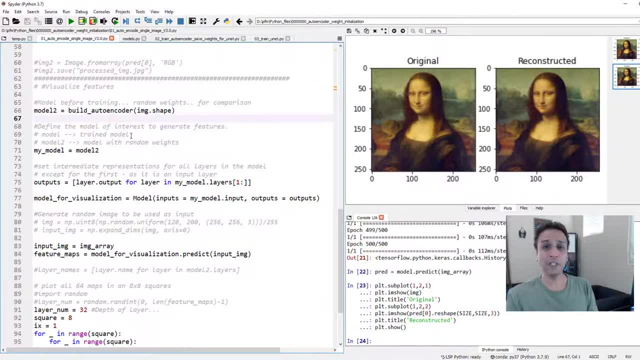 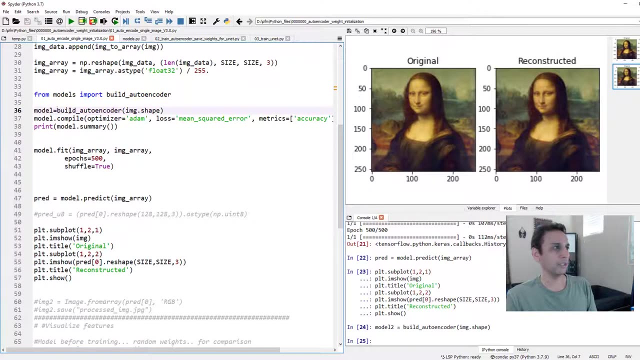 so Let's look at The features. how do you look at the features from your model? so first of all, let's build another model, another auto encoder. so this is basically Remember here. We built a auto encoder Right there, and then we compiled and then we trained. now 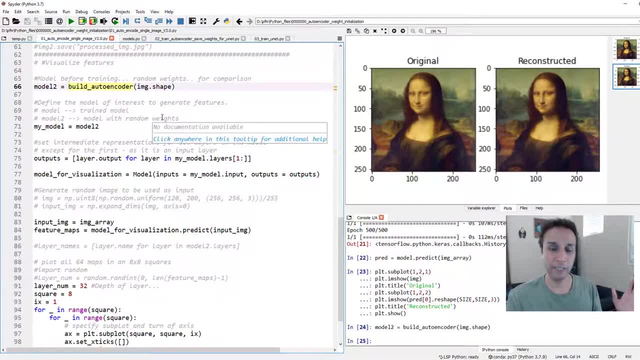 I just want an auto encoder that hasn't been trained, meaning with random weights. Why am I doing this? just so we can look at features before And after. that's it, no other reason. and then I'll put: I'll make my model the current model I want to use as model 2, which we just defined, and 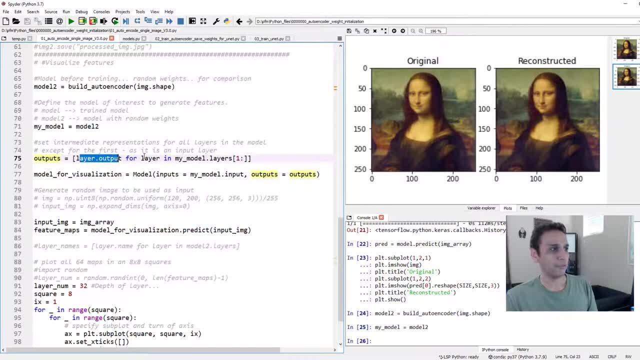 We are going to get our outputs as layer dot output for each layer in my model, Starting with first one- yeah, the 0th one is the input- and then go ahead after the first one. so this Line: when I run it you will see that my outputs right there has. 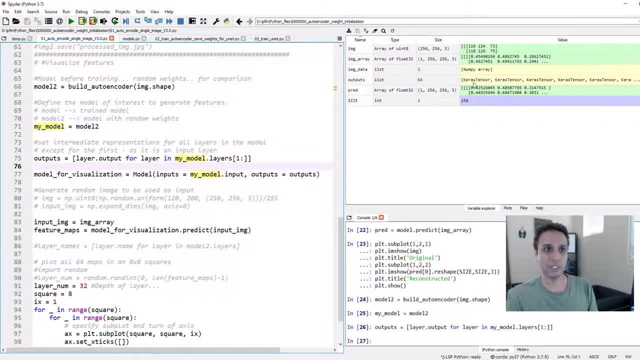 63. size of 63. It's a list of 63 Keras tensors. Okay, These are the 63 layers I have in my auto encoder. Okay, now Let's define a model for visualization, Which is basically my inputs- is nothing but the inputs coming from this model. 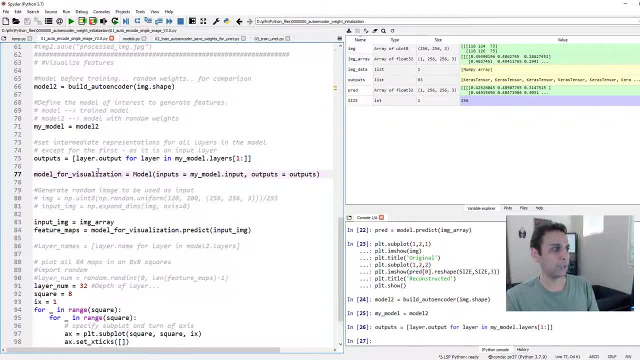 Which is the input or input image, and my outputs is just the outputs that I just defined here, Which means, if you do this, you'll get 63 different outputs, each one corresponding to each layer here, which gives us everything we need For plotting. so let's go ahead and define this model, and we just define the model. we need to predict using that model. 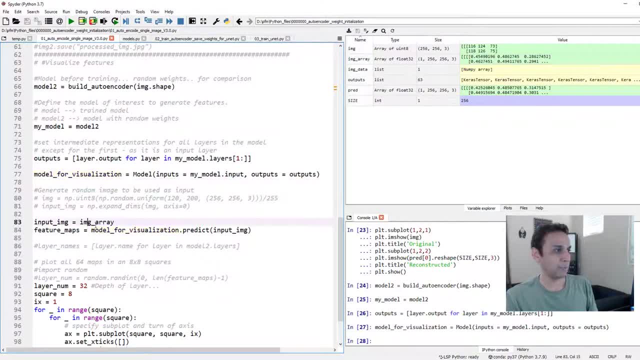 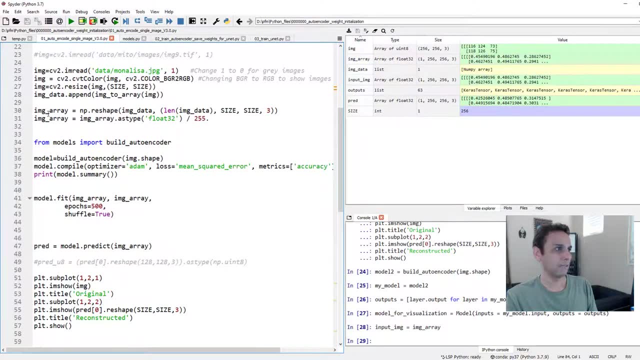 Remember, we haven't trained on this one, right? so let's define. my input image is basically my image array, which we just Did earlier, right? I mean, that's what we called it. Yeah, the Mona Lisa image. and Let's generate our feature maps. feature maps is basically this new model we defined. 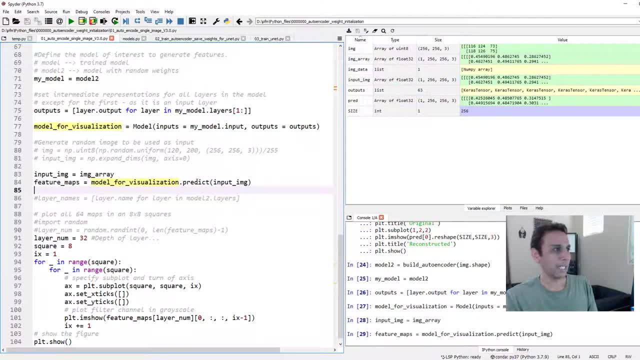 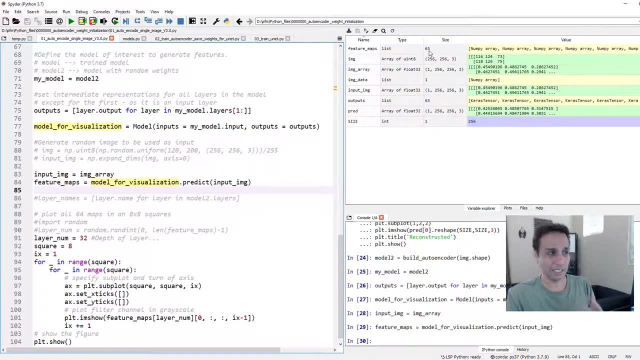 dot predict on my image and When we do that, we should get 63 outputs, hopefully. feature image, feature maps, 63 numpy arrays. Why 63? again, we have 63 layers. That's why we defined our output equal to outputs. We get 63 layers and now I have 63 feature maps. Just pick which one you want to plot. 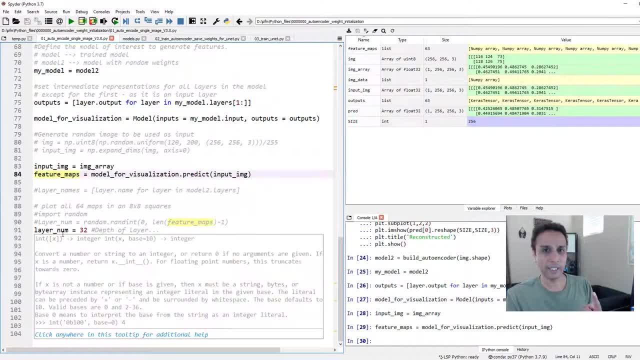 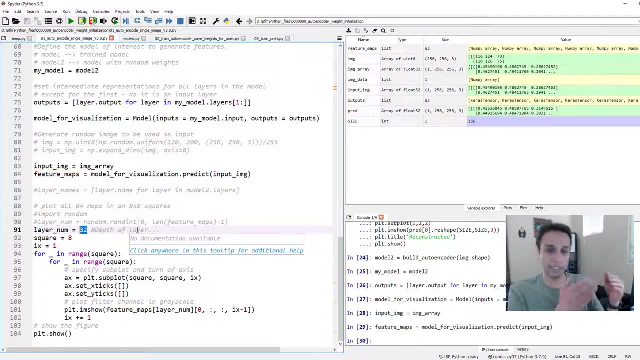 That's exactly what the bottom part does. so let's look at just single layer. I'll share the code. you can experiment with this. Let's look at the last layer, 32nd layer. well, 63rd layer is the last layer, But 32nd layer is the last layer. 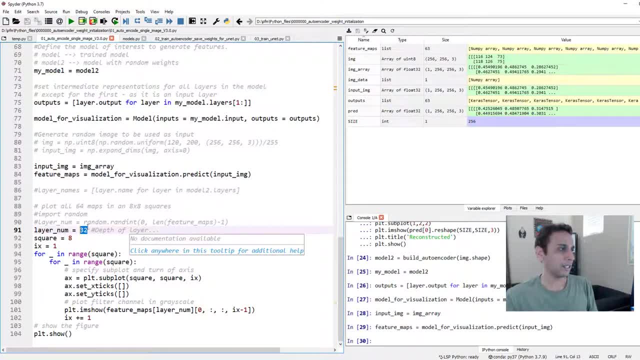 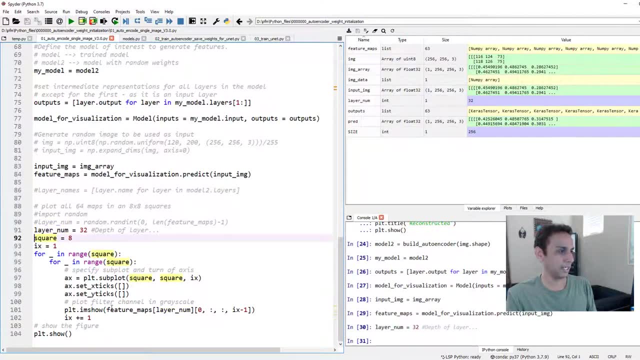 of auto encoder exactly halfway through. okay, so let's look at the layer number 32 and Let's plot my original image and the feature map. okay, right, actually I'm not plotting original image and feature map, Sorry. let's plot each feature maps as a grid of 8 by 8, so we'll get 64 feature maps. 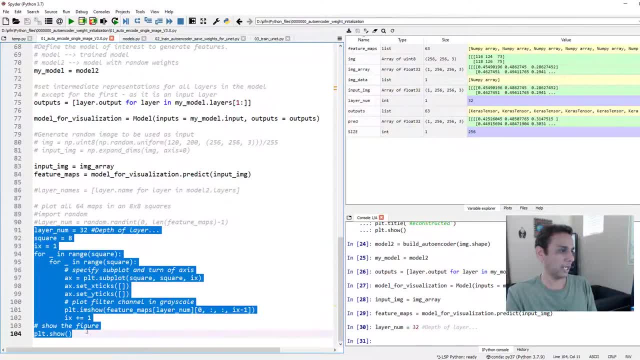 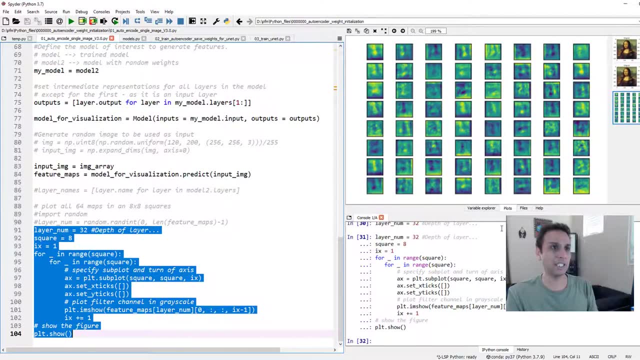 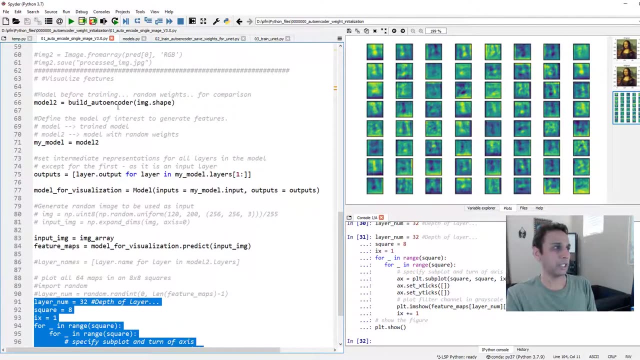 okay, for the layer number 32, so let's go ahead and plot it. and Right now it's predicting. Sorry, it's plotting each one of these. and there you go. I already showed you this as part of the presentation. I just want to make sure you see it live, and this is based on. 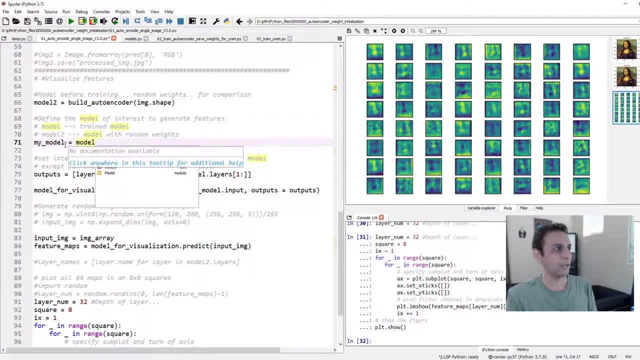 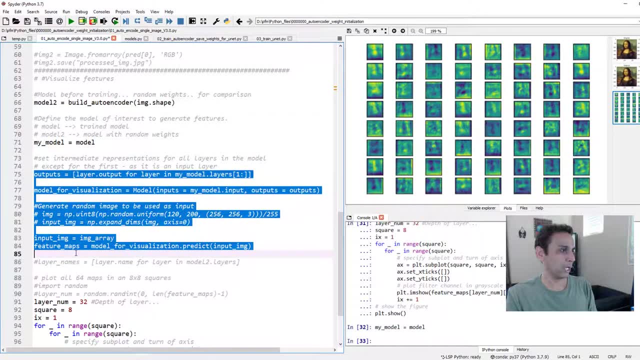 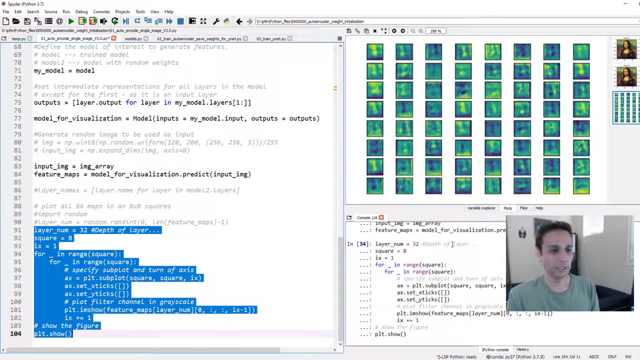 random Weights. now let's use the trained weights. How does the you know the feature maps? How do they look like? so let's go ahead and run all of these lines and then finally plot them. once we have it, go ahead and plot it and 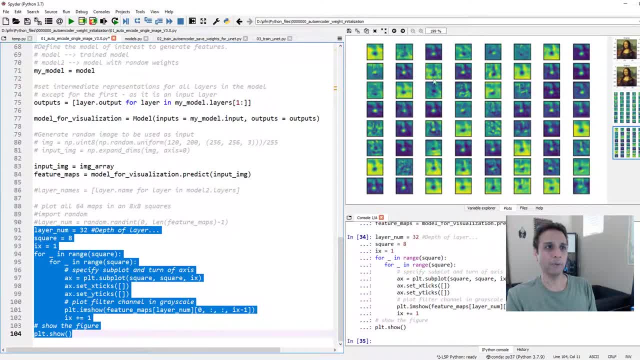 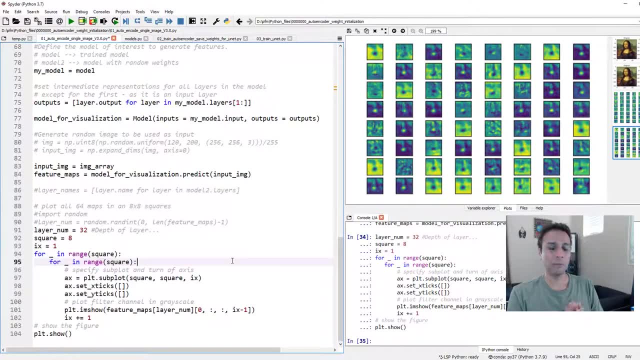 And hopefully we should see some structure there. you go nice structures right there, okay, So I hope you got the point of using are the benefits of Pre-trained models? now you can use, for example, the ImageNet weights. that definitely helps. This is what we call transfer learning, but ImageNet is a bunch of animals and trucks and these type of things, right.